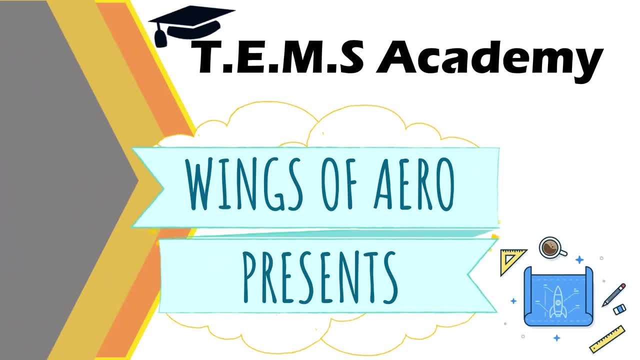 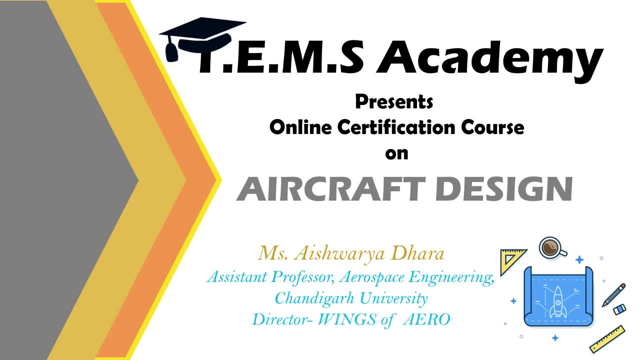 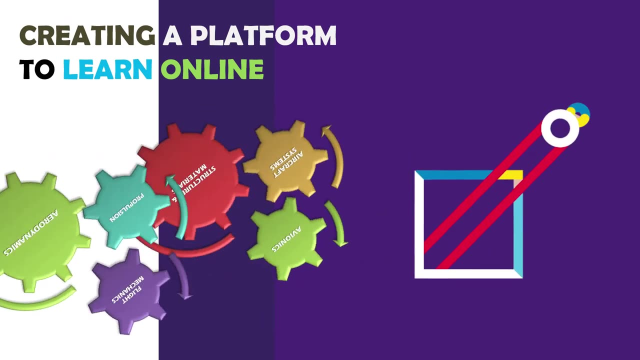 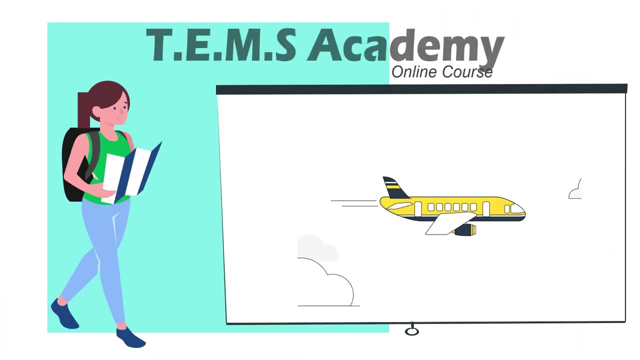 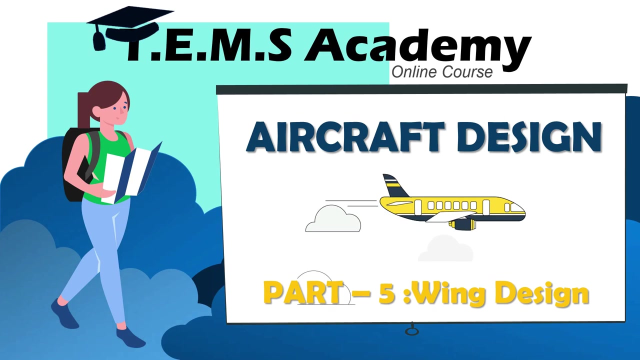 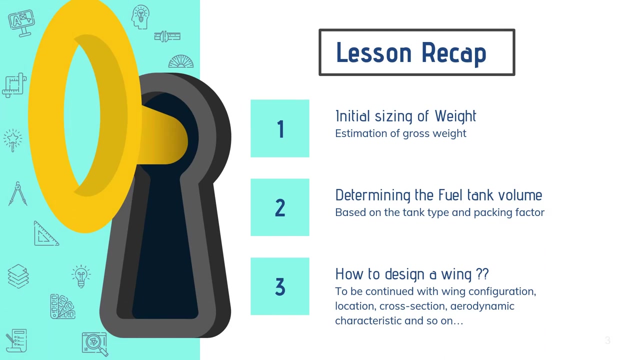 Hi friends, welcome to Aircraft Design Model 5- Wing Design of an Aircraft. Without wing, aircraft cannot fly, which is the critical part used for lifting, turning, landing and controlling of the airplane. In the previous module you have learnt about the initial sizing of the aircraft's weight and calculating. 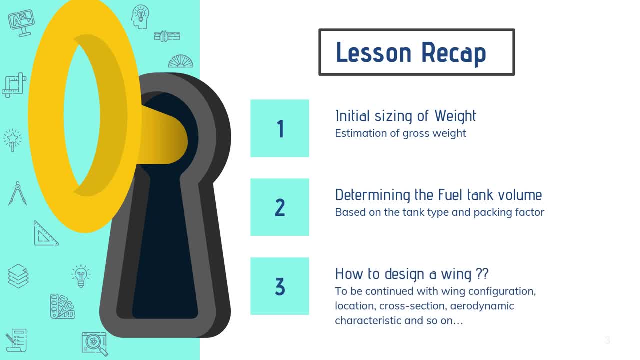 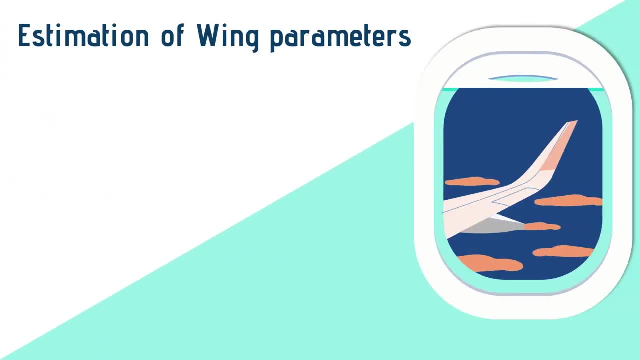 the fuel tank volume. Now, in this module, you will learn how to design a wing of your aircraft based on federal and military aviation regulations, For various aerodynamic considerations. it starts with selection of wing configuration, with various platform, number of wings and its location, Then estimation of aerodynamic. 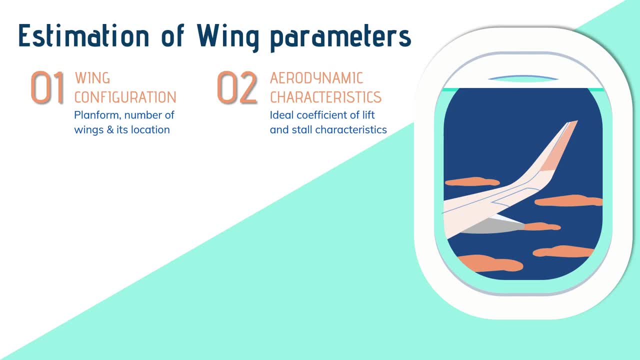 coefficient of an airfoil which will satisfy the following: airfoil width and thickness to chord ratio, Then followed with wing parameters like aspect ratio, wing area, span, taper ratio, Mean aerodynamic chord, then swap angle, twist angle, incident angle and dehydral angle to 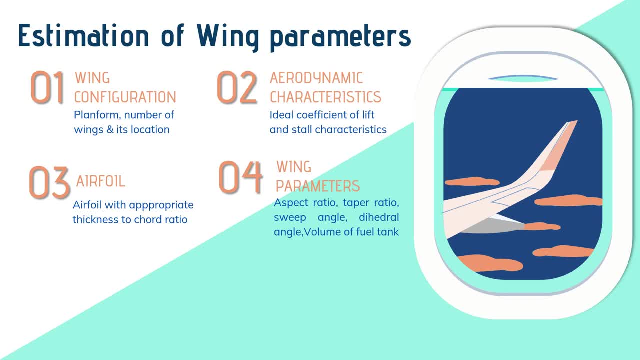 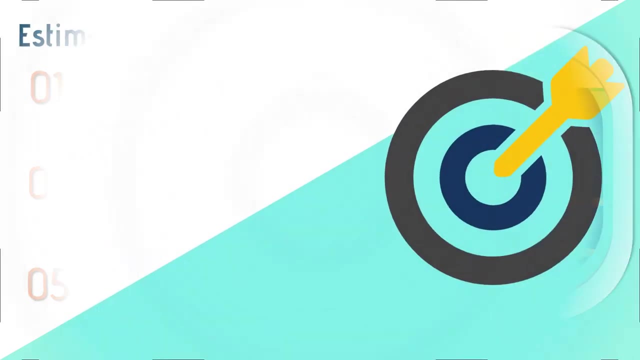 satisfy the fuel tank volume. Then you will also learn about the high lifting device and its application, And finally you will calculate the lift force obtained during takeoff, landing and cruise. So this video can extend a bit long. Stay tuned till the end of the lecture. 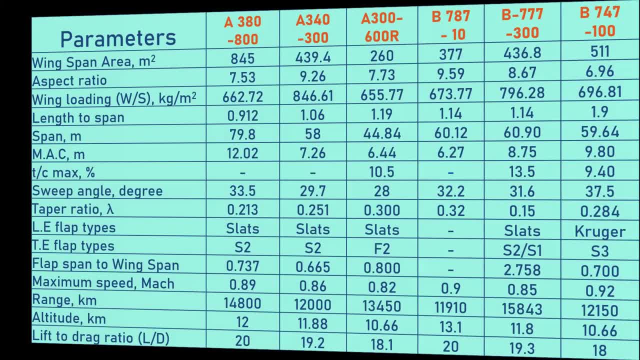 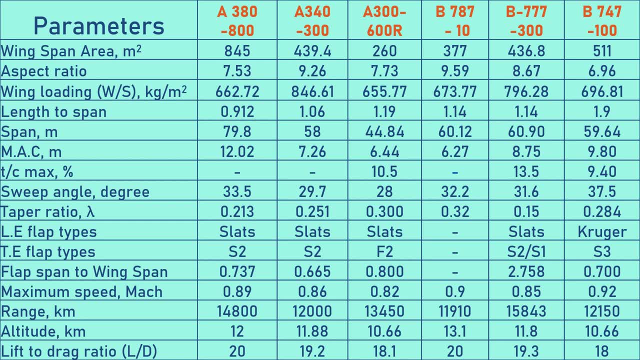 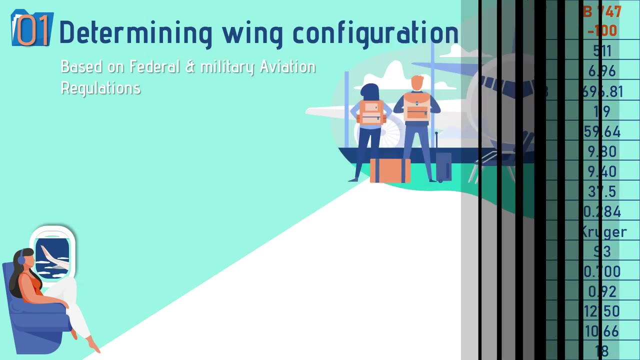 and definitely you will gain knowledge from it. So, before proceeding, here is my wing configuration data for a large passenger aircraft, wherein each phases I will give you the demonstration how to do a wing design and obtain the parameters with justification, And similarly you can proceed for your design. 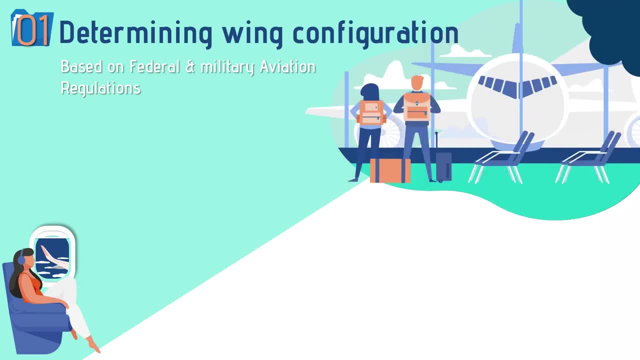 So we will start with. based on federal and military aviation regulations. It is based on the design of the aircraft. It is highly desirable to predict the maximum lift coefficient and the stalling characteristics of an any aircraft in the design phase. So, starting with the selection of wing platform, it is a top viewed layout or the shape of a wing. 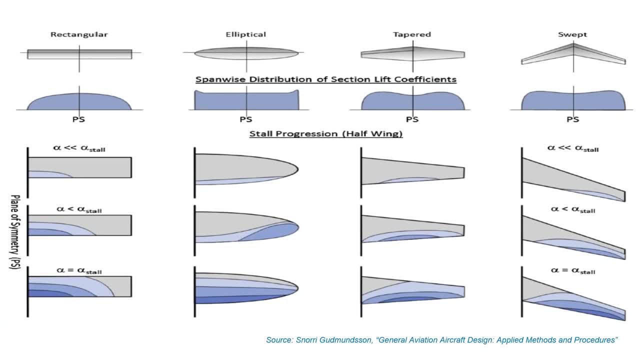 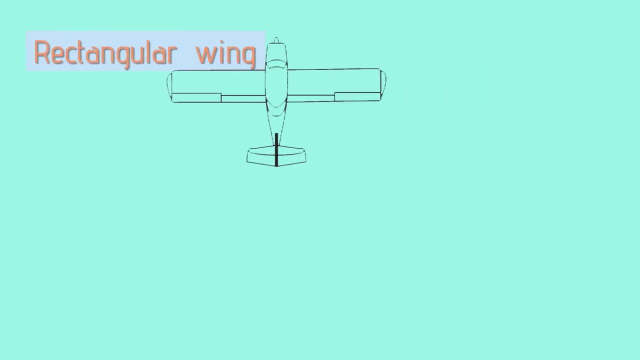 So which influences the aerodynamic characteristics like stall, progression and performance of the aircraft. So basically, there are four platforms: rectangular, elliptical, tapered and swept. First is the rectangular wing- Rectangular wing- it is an excellent from a manufacturing point of view- is a straight and untappered wing mostly used for small. 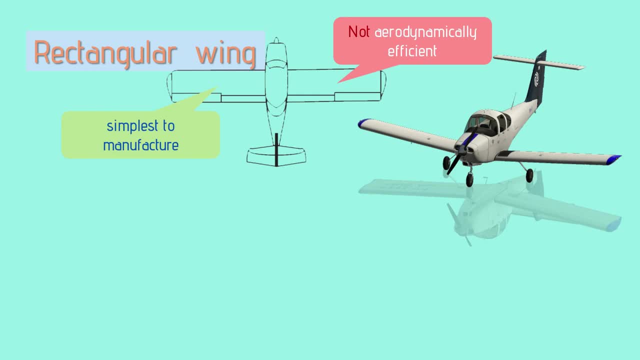 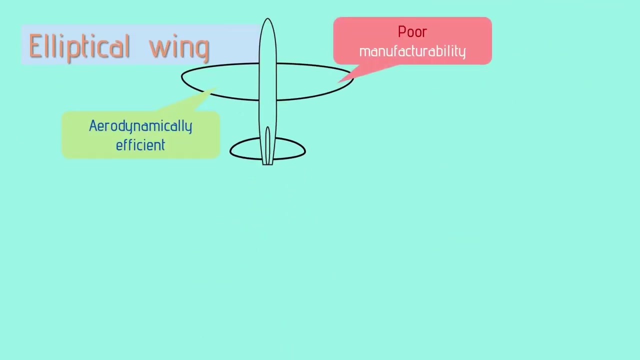 elite general aircraft, like people 38,, but it doesn't provide aerodynamically efficient one. But in case of elliptical it has basically of two types: elliptical and semi elliptical. It is just a reverse of rectangular wing Which is aerodynamically more efficient but poor from a manufacturing point of view. 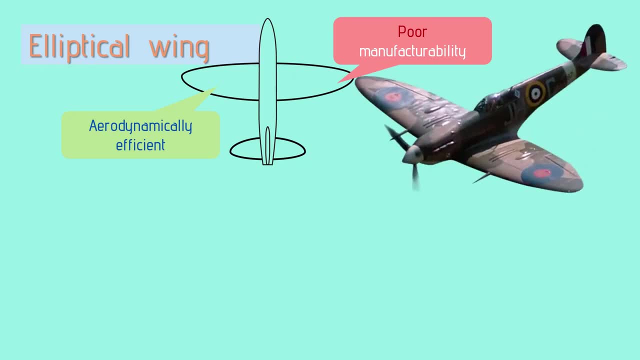 But the most significant example is a speed fire. It aimed not only to minimize the drag, but also create a house for landing gear, along with an armature and guns inside a wing. Next comes Tapper wing. Tapper wing are basically of four types. One is a Tapper- reverse Tapper. 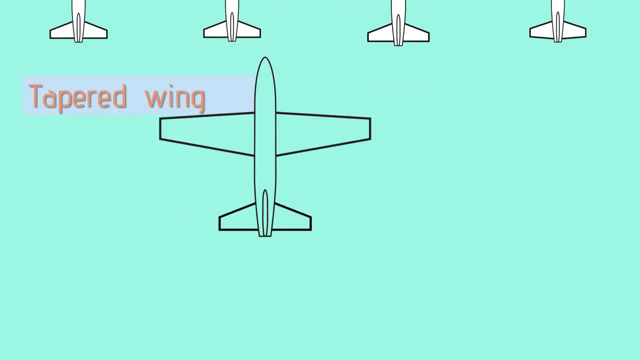 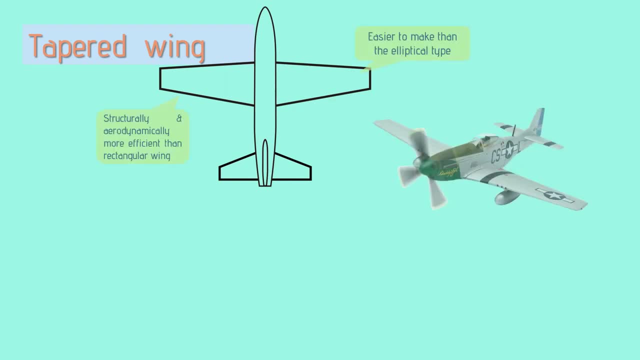 compound Tapper and Tapper outboard. So Tapper wing is a modified version of rectangular wing which is a line between moderate efficiency and moderate manufacturability. Under this swept, Tapper wing provides an outstanding performance at a high speed flight Trailing. 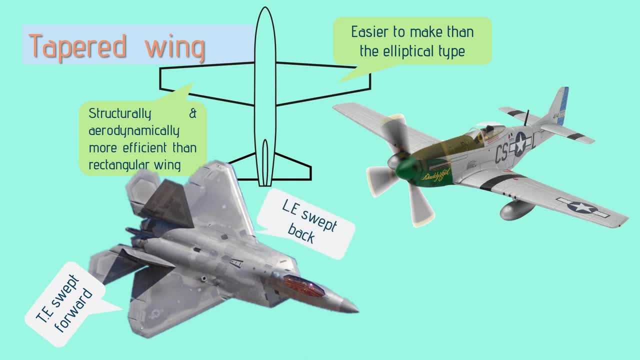 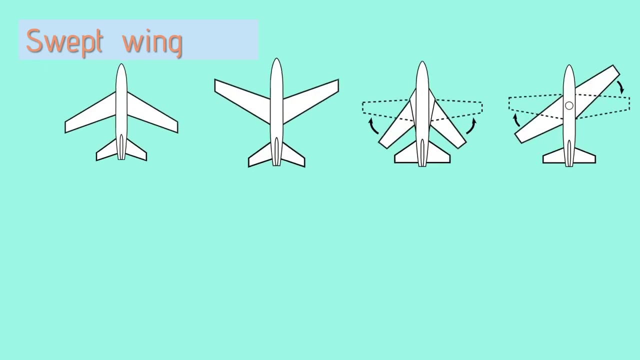 edge of the wing swept forward and the landing edge swept backward. The most well-known combat aircraft is the Martin Raptor 22A. Next is Swept back- Swept back, having another four types: Swept back wing: swept forward, variable swept and variable oblique wing. The swept back wing does leading edge a swept. 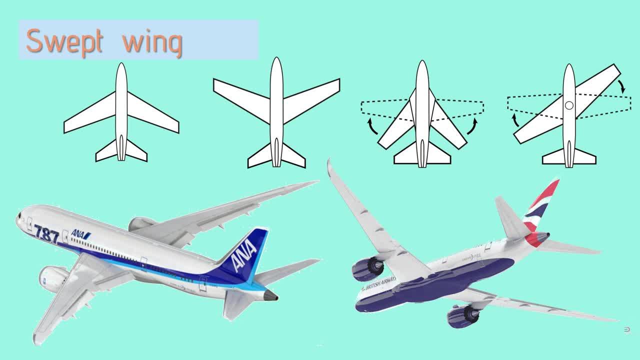 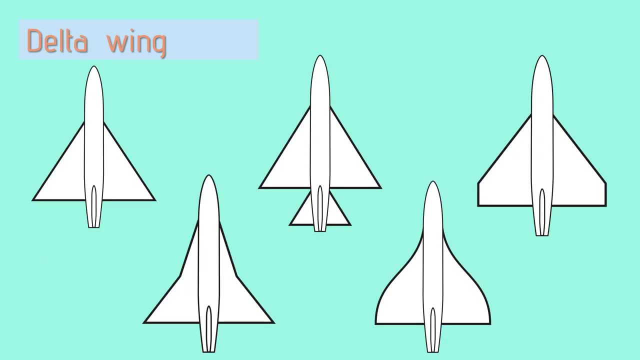 backward to reduce the drag and win the aircraft flying at transonic speed, like Boeing, Airbus, passenger aircrafts. Now, one more specific type of wing is a delta wing. There are five kinds of Delta wings. Delta wing are mostly pasta wing, tail, wing tail. 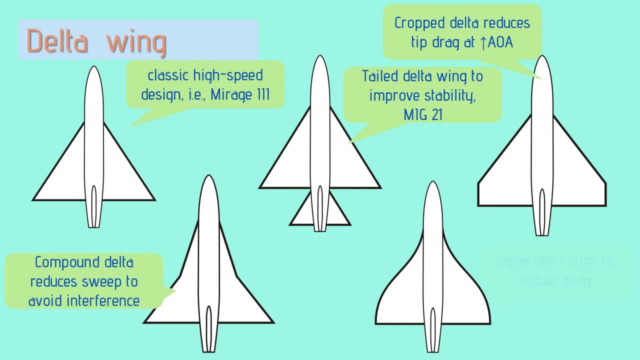 wing delta, wing delta, tucking and tail wing. Then we have tail delta, wing, crop delta and cap delta. Next, Coming up from baiting, Delta wing Delta, wing Wins Delta wing stands up to another five types. One is Taleless Delta. 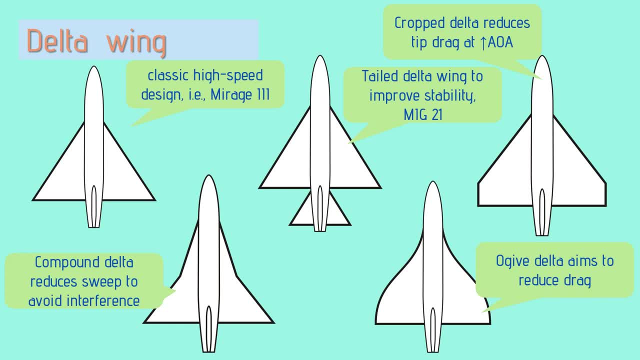 Delta wing is also known as a Agile wing and Double delta wing, Grop delta and Delta jump delta. Delta wing is a simular to Ajaib wing. swept wings are the delta wing. please make a note of that. so based on your design criteria, please. 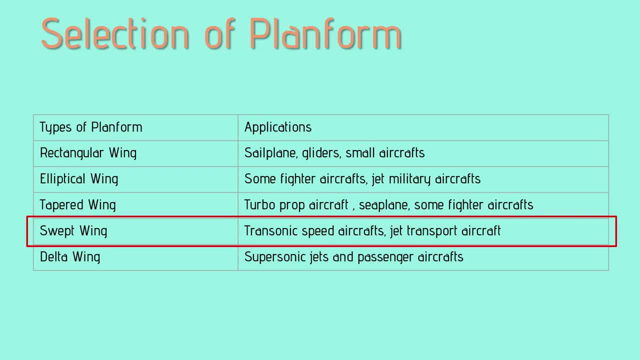 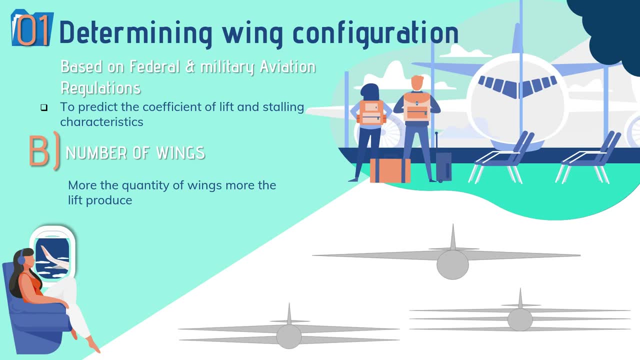 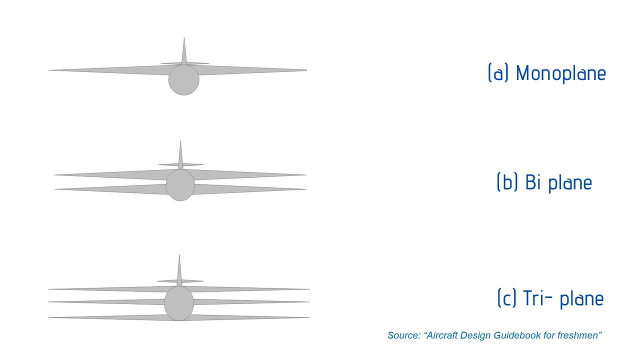 select the type of wing platform coming to the next is the number of wings. that depends on the designer, basically of three types: monoplane, biplane and triplane wing. so, based on the principle that more the number of surface area, which helps to pressure exerted, more on the surface and hence 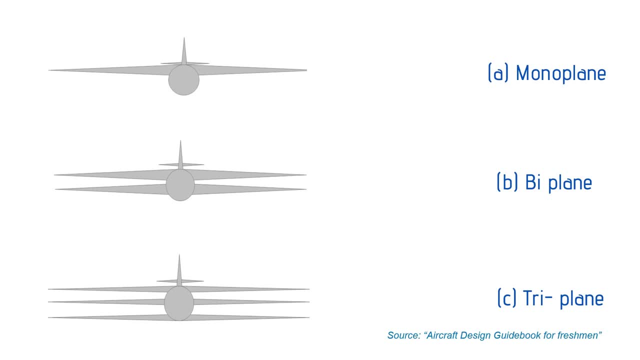 generate more amount of lift. in addition, it's also create the more amount of interference. drag triplane as an fokker, biplane as a ride brothers and monoplane aircrafts like commercial- any aircrafts, though mostly monoplanes, is preferred at the current scenario to reduce the interference. 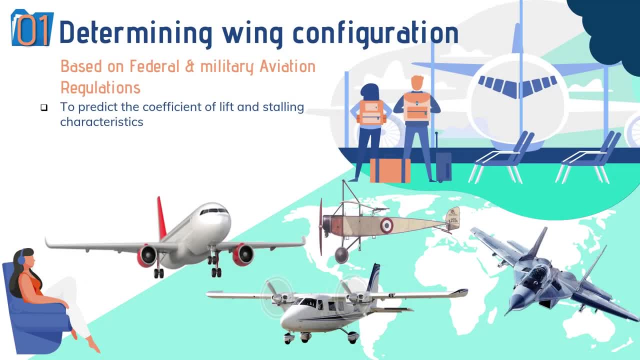 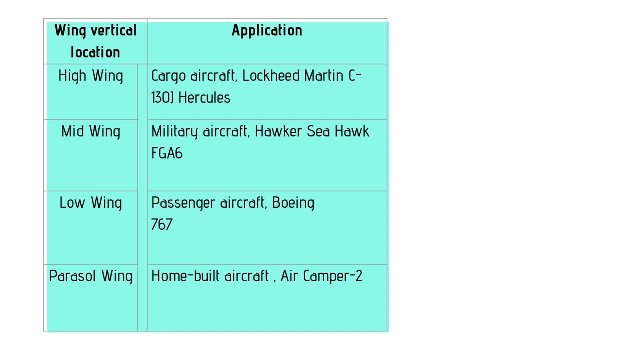 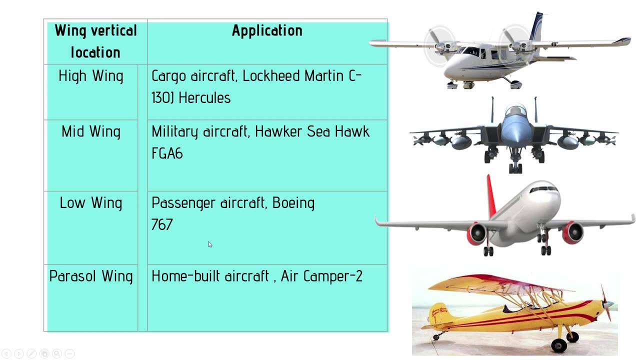 drag monoplane with maybe monoplane wing, may be mounted at various positions relative to the fuselage, like high wing, mid wing, low wing, parasol wing. so based on the purpose of the aircraft, as shown that that most of the cargo aircraft is configured with high wing fighter aircraft with the mid wing large passenger aircraft. 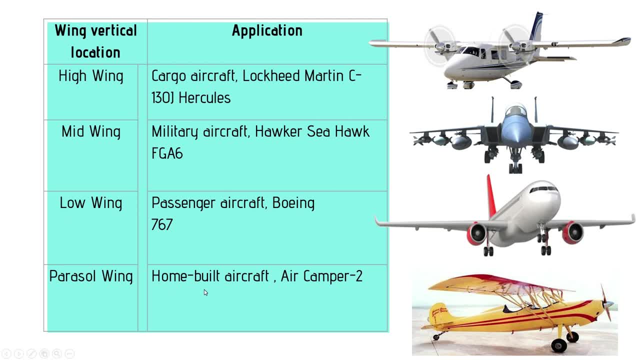 configured with low wing configuration and parasol with an ultimate light aircraft or the ultra light aircraft, home build etc. are configured with a parasol wing. to know more about the effects of the configuration, link is in the description box. to satisfy the fuel tank volume, let's to choose the 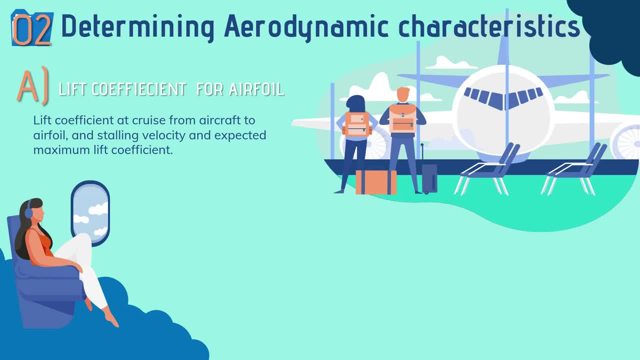 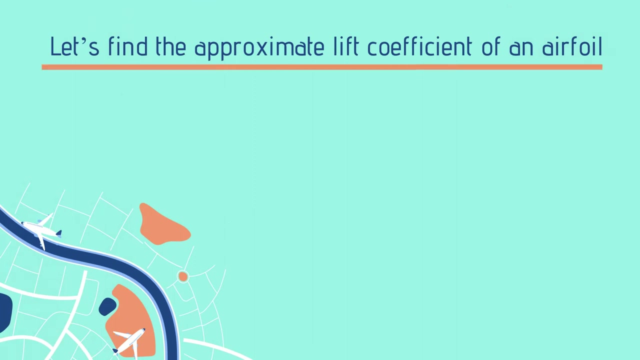 thickness of the wing section, which involves choosing the airfoil with respect to correspondent flight velocity. now, selection of airfoil also depends on lift coefficient, aerodynamic efficiency, movement coefficient, other parameters like wing area, swipe angle, Etc. so let's find the approximate proportion of an airfoil now, recalling the steady level flight, that is, lift equals to weight, so 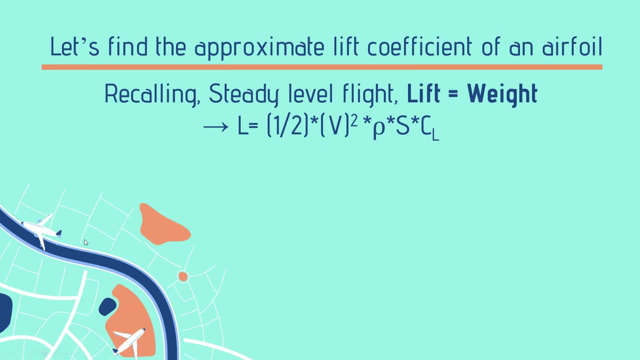 lift equals to half row V square Rho s cl. now at the cruise to find out, the cruise velocity equals to some amount of maximum velocity. mostly it is 90 to 96 percentage. so let's consider the 90 percentage. that is, cruise velocity equals to 0.9 into vmax. now, after substituting, the vmax is: 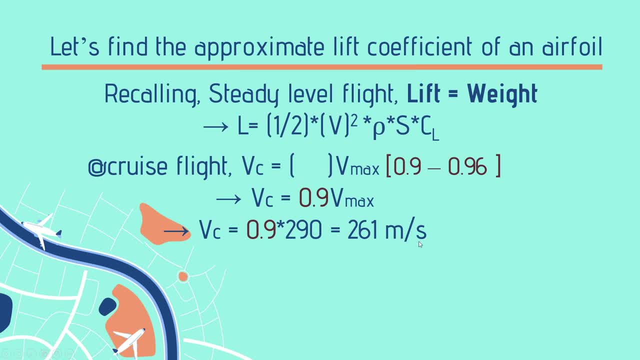 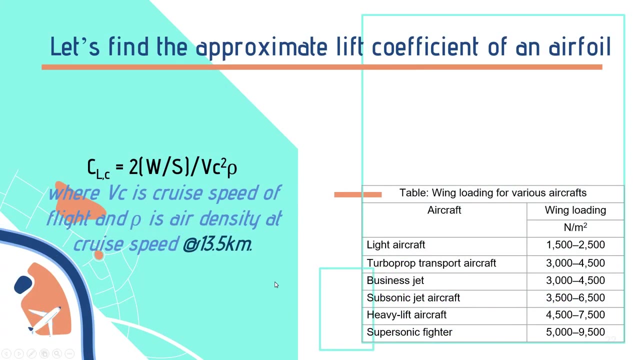 290 for our design criteria, then i have got. 261 meter per second is my cruise velocity of my design flight. then substituting the values in this cl basic lift coefficient of a wing of an entire aircraft, that is, density at the cruise altitude. now here we have considered: 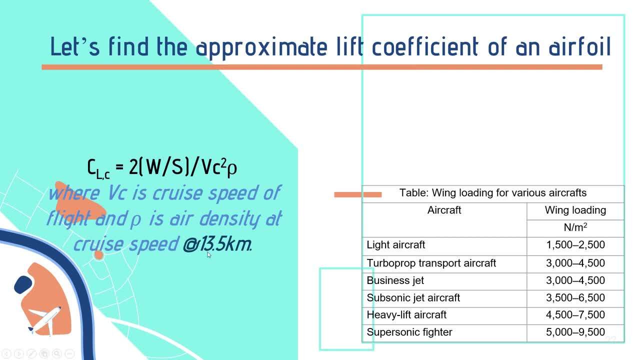 the cruise altitude as 13.5 kilometer. so at that particular altitude the density becomes 0.246 kg per meter cube. now here in case of wing loading cross, check the value here. our wing loading was 750 kg per meter square. now convert that in newton per meter square, as you can see. 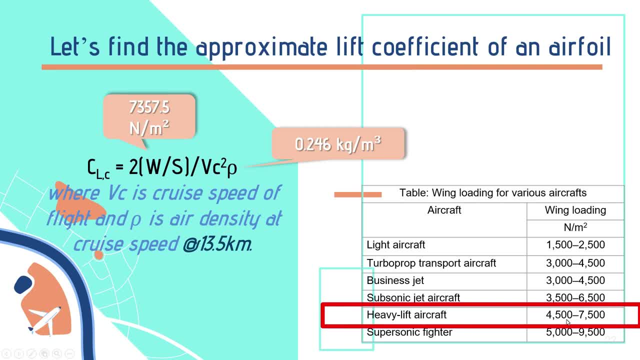 in the table for an our aircraft. it produce the range between 4500 to 7500 newton per meter square. now if i calculate our parameters, that 750 into 9.81 to obtain newton per meter square, we get as 7357.5 newton per meter square, and which is a proper limit. 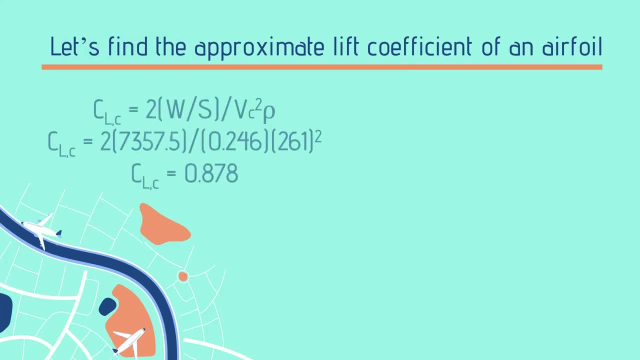 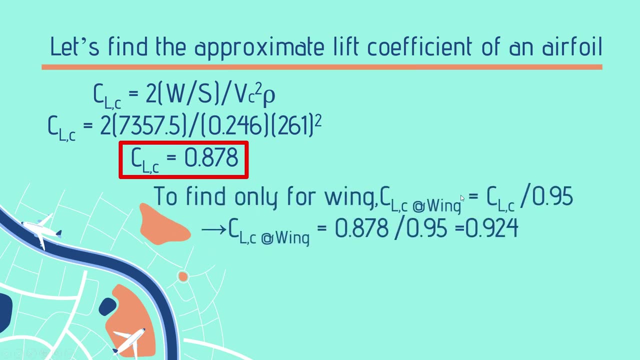 now substituting back and we get that cl cruise becomes 0.878. now to find for wing alone, the cl, then we are going to divide that cl of the aircraft at the cruise by 0.95. after that we get 0.924. now further calculating that to find for the airfoil. 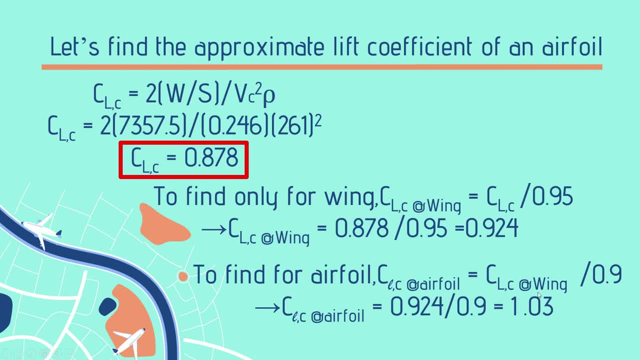 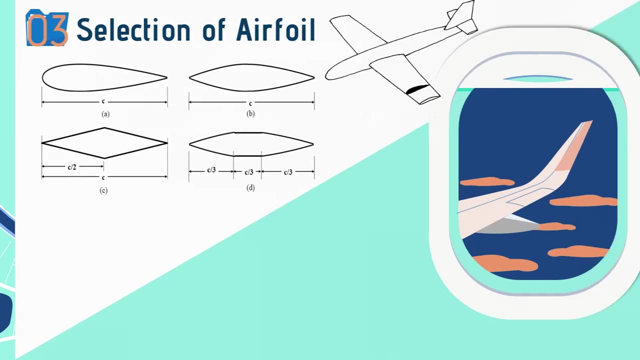 clc at for airfoil for the cruise be divided by 0.9, we get 0.924. by 0.9 becomes 1.03. now, based on this parameter, we are going to find a airfoil, one of the most important parameters in designing. 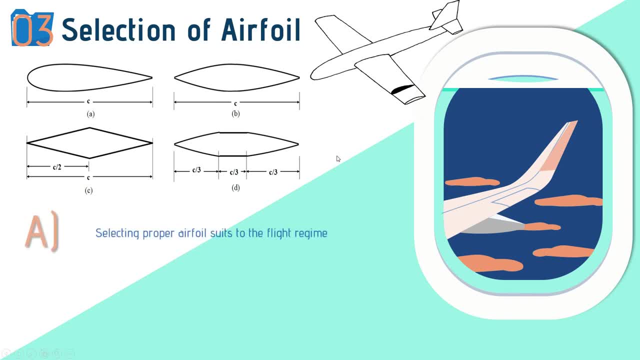 wing of an aircraft is selecting a proper airfoil, so it's for an flight speed, a drone in figure in this aircraft selection can be performed based on the aircraft speed and the requirements can be picked from the following figure. as you can see the figure a from the 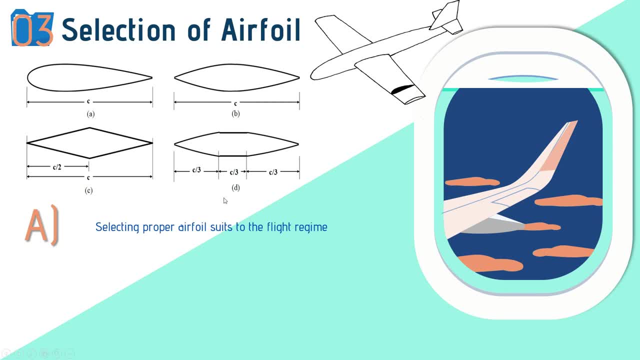 figure a will be suitable for the subsonic flight and from the b, c and d is suitable for the supersonic or high speed aircrafts. so based on that particular profile, you have to select an airfoil. next comes the airfoil. thickness ratio has an important or impact on the drag lift coefficient. strolling: 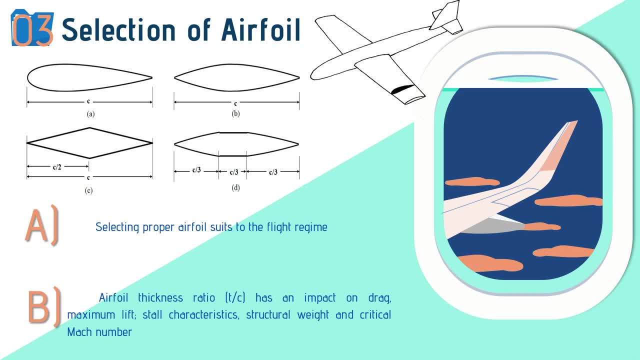 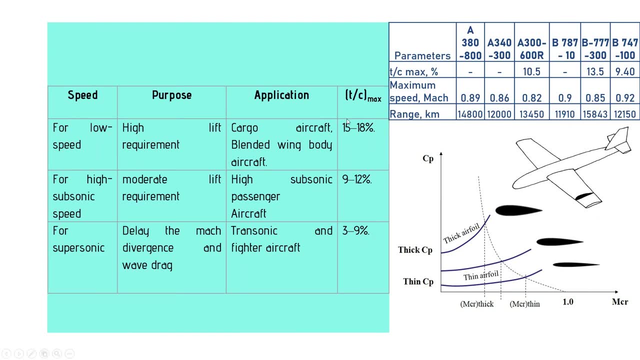 characteristics, structural weight and critical mac number. as per the thumb rule, typically the values for an airfoil maximum thickness to core ratio of an aircraft ranges between 3 to 18 percentage, as you can see in the table. for your kind guidance, you can refer that for a low speed. 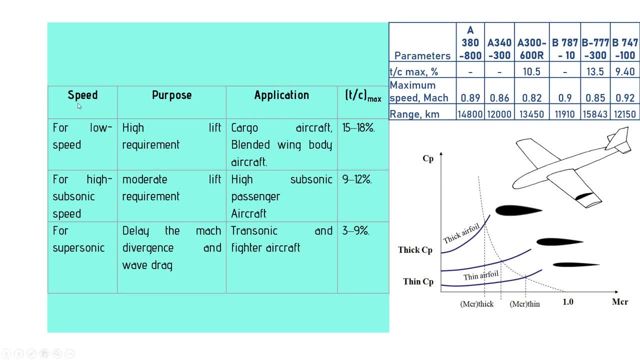 with an high lift requirement, like that is cargo which thickness to core ratio maximum ranges between 15 percent to 18 percentage, whereas for high-speed aircraft or transonic speed, in which ranges from high subsonic passengers the the thickness to core ratio ranging between 9 to 12, and for the supersonic it. 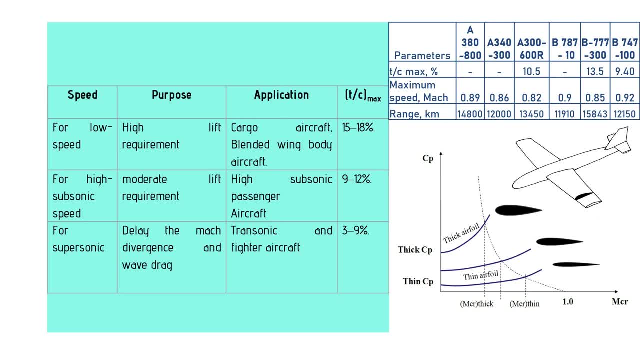 become is 3 to 9 percentage. now if you see the comparative data for my large passenger aircraft, the thickness to core ratio should range from 9 to 12.. diagram- the graph follows 9 to 12 percentage. so if the wing is desired for high subsonic passenger aircraft, select the 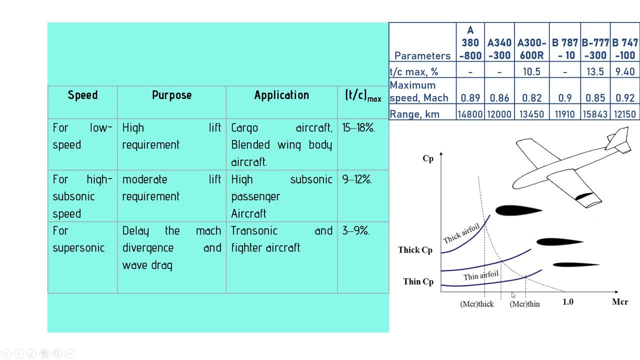 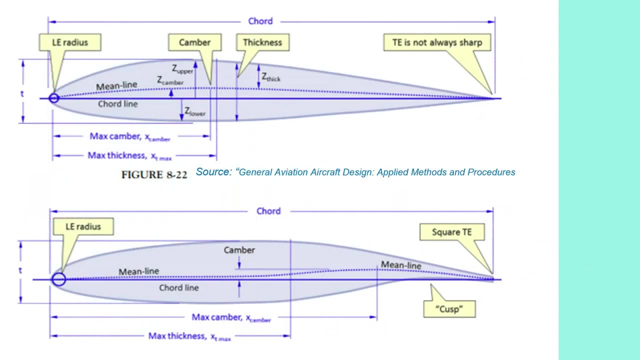 thinnest airfoil. the reason is to choose or to reduce the critical mach number and drag divergence mach number. as the graph shows, thinner airfoil will have the high critical mach number than the thicker airfoil. okay, so these are the basic nomenclatures of an airfoil. there are several. 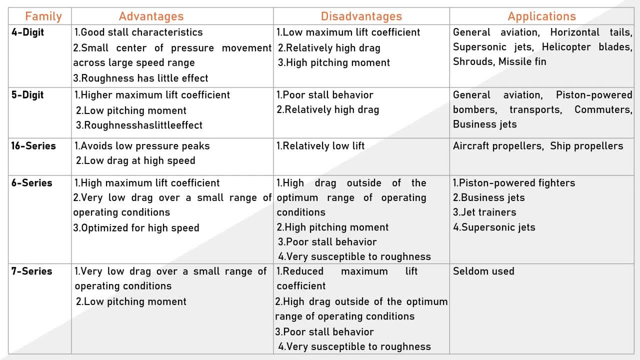 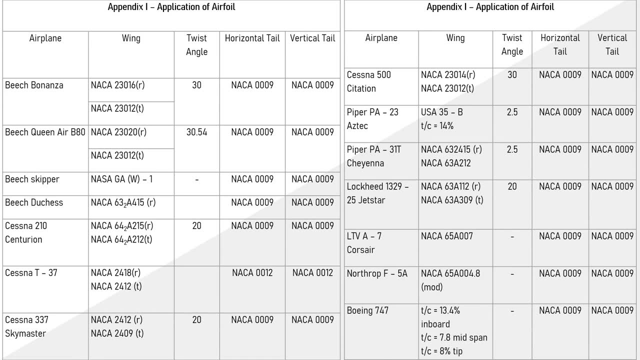 airfoil series. each series have its own advantages and disadvantages. based on the application, select the your own series. after selecting the appropriate series, you can see for business state, for aircraft, for large passenger aircraft, for fighters, which series is preferable now. after that, according to me, i prefer the thinnest airfoil and i prefer the thicker airfoil. 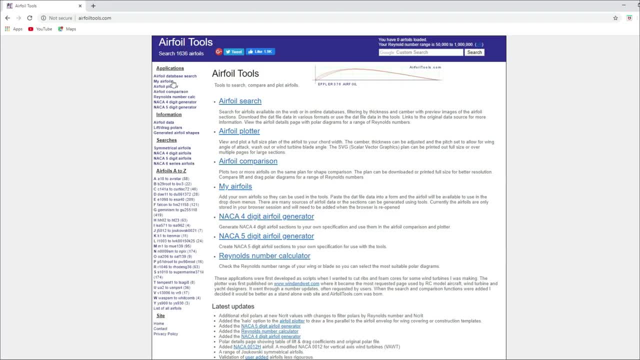 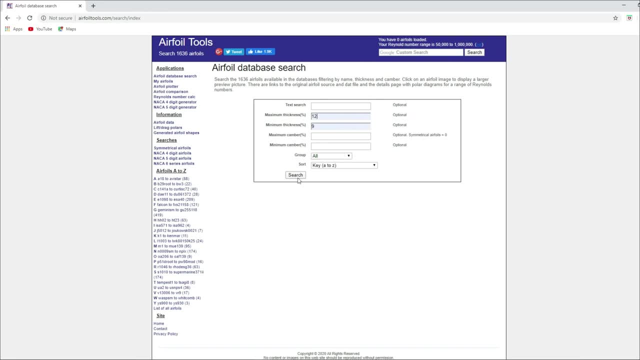 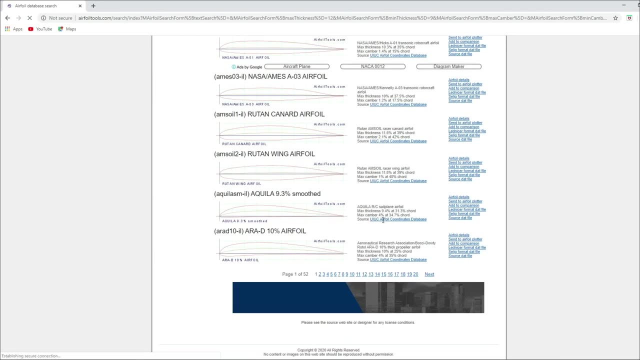 so i will go open an airfoil tool website from there. i will give the minimum minimum thickness is 9 and the maximum is 12, and i will prefer for all sort of airfoils. now here is my sample airfoils. so many sample airfoils are coming up now based on the sample. 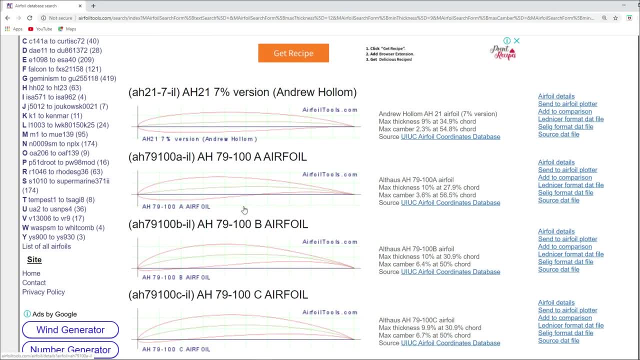 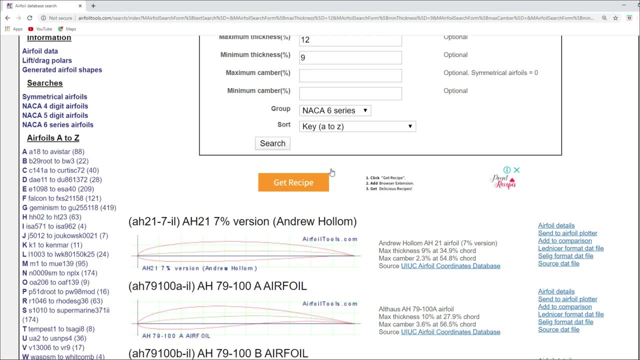 airfoils. i will pick the best one for me because our criteria was 1.03. so i will go open an airfoil tool website from there. i will give the minimum minimum thickness value and based on that particular value, i will try to take a higher than that particular value. 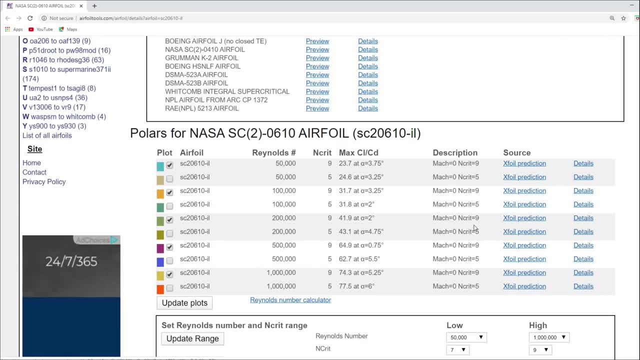 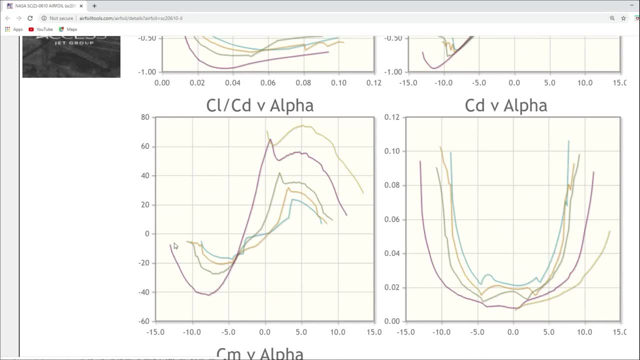 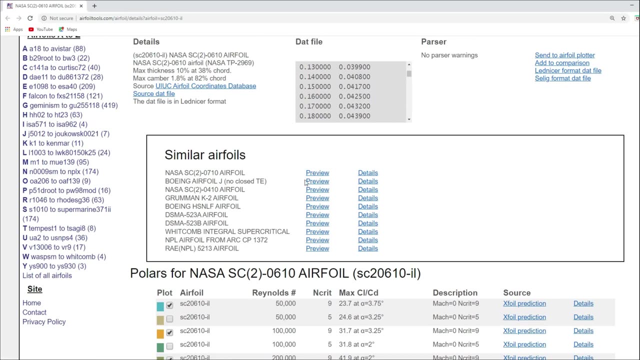 and i will also check that angle of attack, of stall, stalling, angle of attack. so based on such criteria- the thickness, stalling angle and the cl which is opted, so based on this criteria, i will pick the best five airfoil. so you can see here i have picked the best five airfoil now initially, 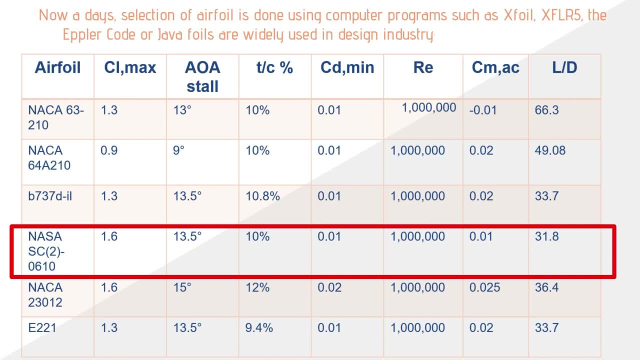 what i will do is i will the best one i find is the best one, which is the best one, which is the top lane cl, then i will pick that one. this naka23010, i will go there and my seconds are: first is my fifth one and my 904 at the top, Qiuquai is the third and my sixth one is: 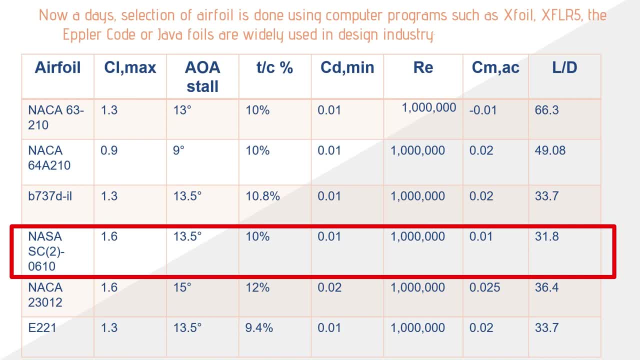 naka23010, and my sheet is naka230. Geoffrey, ruling 26.9. here is nasa sc2: 0, 6, 1, 0, and second one is a naca2301. to now, from here though, this naca23012 have a 15. 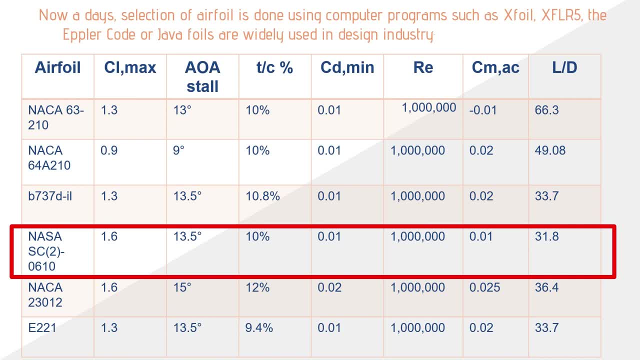 degree stalling angle, but it has an thickness to core ratio 12.. i don't want. i will proceed for the next. now see: nowadays, selection of airfoil is done using computer programs such as xfoil, xfl, r5- there are so many are widely used in the design industries. 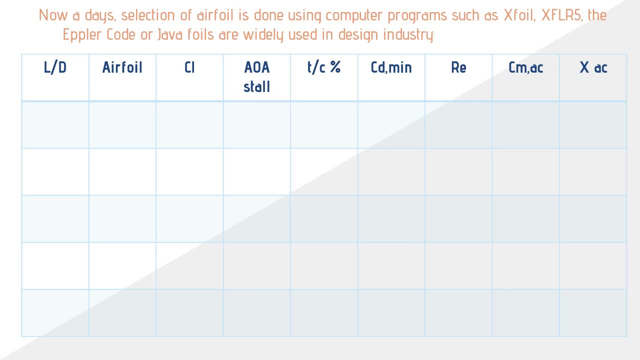 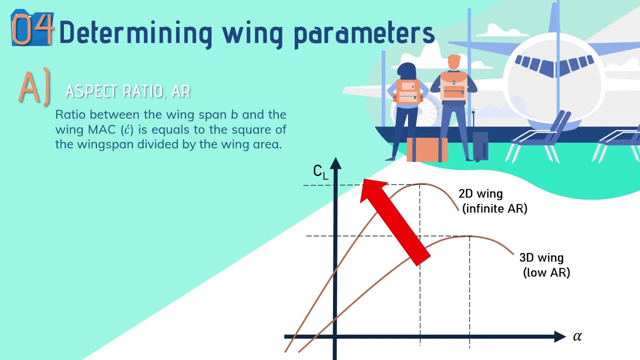 so, according to your design, you can also modify your tabular column like this. also, you can find your l by d. accordingly, you can find the airfoil and satisfy the other criterias. now, moving to the aspect ratio. aspect ratio is the ratio between the square of span. 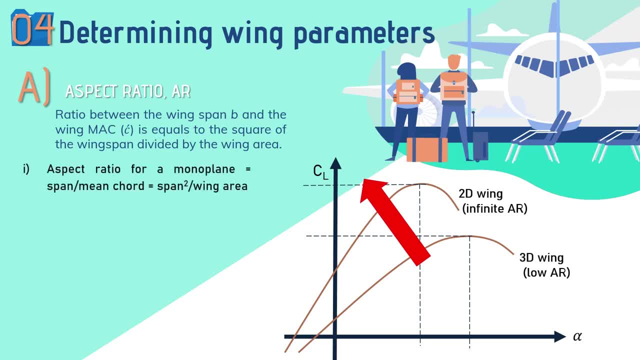 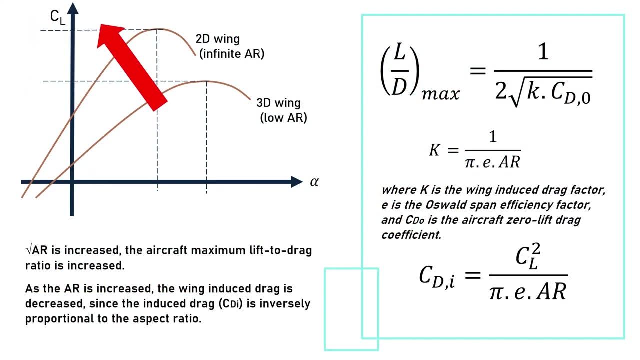 by the wing area. so based on the type of number of wings, the aspect ratio will also vary. for monoplane, the aspect ratio is a b square by ace. for biplane: 2b square by ace. triplane: 3b square by s. to know more about the aspect ratio on an aircraft, link is in the description. 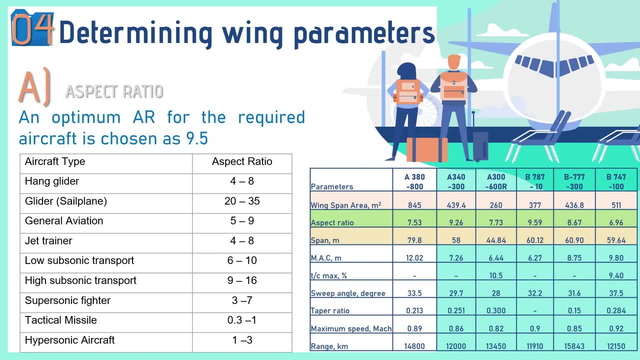 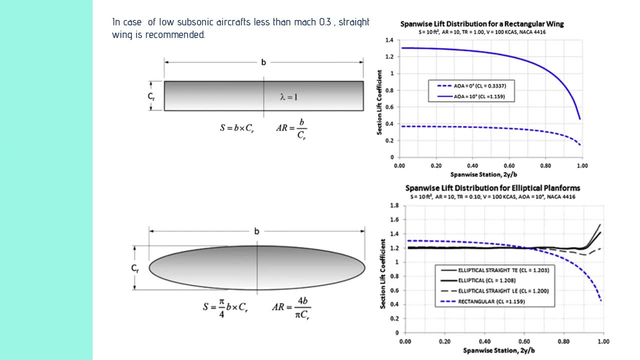 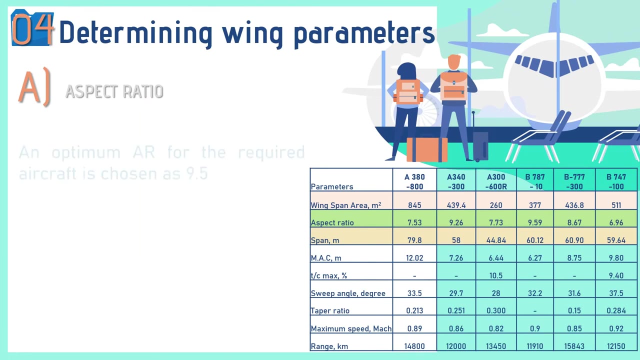 box. so from the table it is clear that more the speed, less the value for the aspect ratio, which helps for better maneuver. uh, based on your type of aircraft, you need to select the particular platform. now, coming to an using the optimized value for an wing loading that is, 750 kg per. 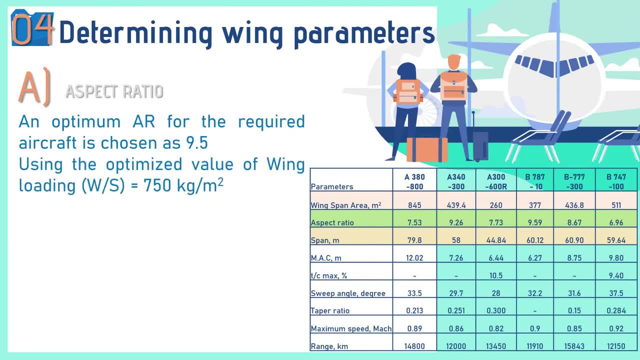 meter square. now we need to obtain the wing area, so the area can be written as wt0 by wing loading. so, whereas the wt0 becomes 331787.610, which we have obtained from weight estimation, divided by the swing loading that we have optimized, that is, 750 kg per meter square. 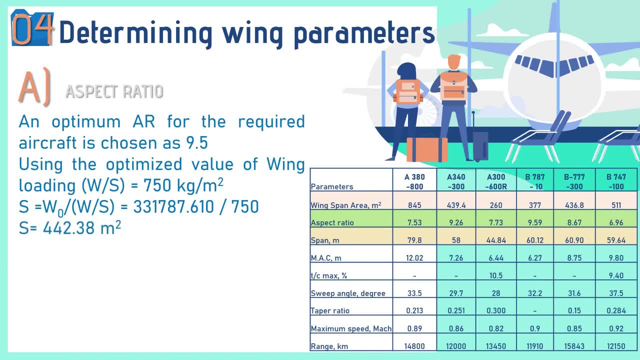 now substituting the value, we get. that value of wing area is about 442.38 meter square. now to obtain the wingspan, recalling the aspect ratio of the wing area, we need to obtain the wing area by recalling the aspect ratio. aspect ratio, we have chosen 9.5. so aspect ratio equals to b squared by. 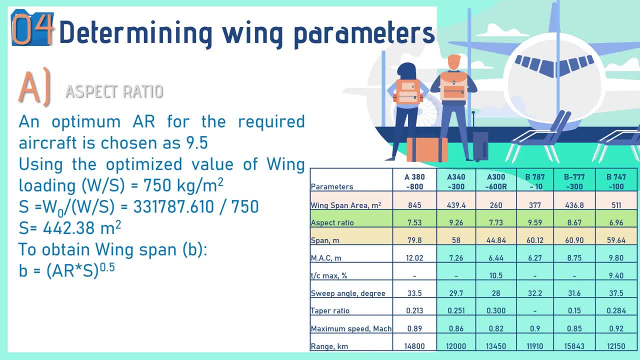 s. so b becomes root over a r into s. substituting the value that is 9.5 into 442.83 and resolving, we get as 64.81 meter. that is a span length. wing span length coming to the next is a tapper ratio. 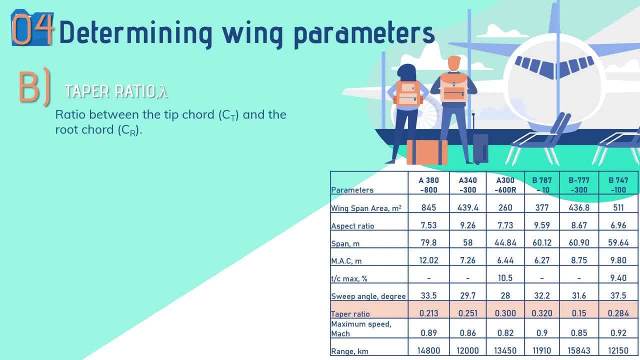 tapper ratio is an ratio between wing celebrate length and wingspan length. the entire positioning is: Он переш Sydney dangerlation. the total length: 이 난 lö viewao middicum. we plan after Wiring zone property control is all that is light minimum, the tip chord to the root chord. so basically, tapper ratio denoted by the terms lambda, which 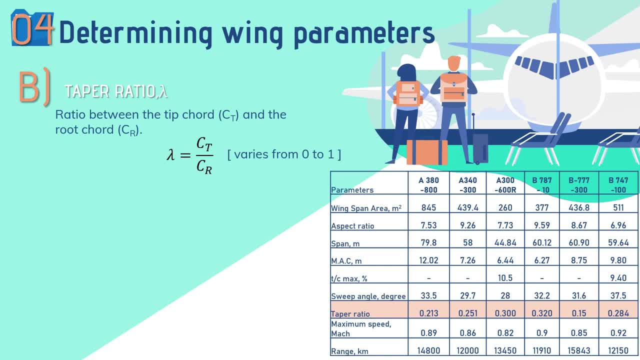 is ranges between 0 to 1, and tapper ratio plays a very important role in an induced rack structural width and fabrication point of view. now considering the induced rack. the induced rack gets lower for a tapper ratio between 0.3 to 0.5 if the tapper ratio that 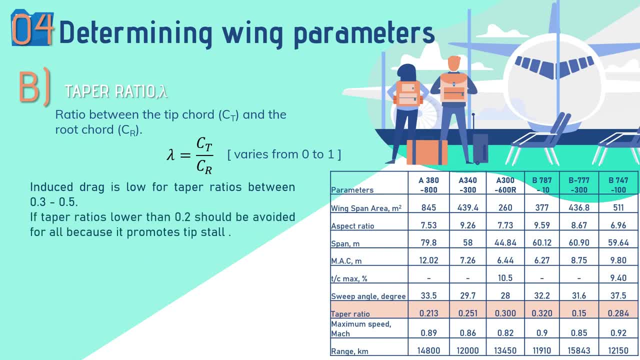 is lower than 0.2 should be avoided for all because it's promote tip stalling. so considering that. so again comparing the comparative data study for an large passenger aircraft here you can see the tapper ratio varies from aircraft to aircraft, so you can see it is also ranging. 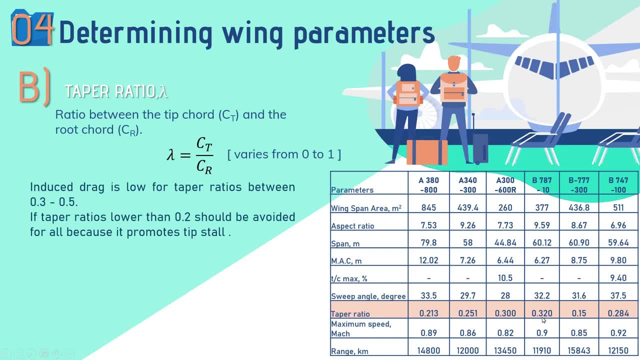 between 0.15 to 0.320.. so, as we know that it helps to reduce the induced rack when it is between 0.3 to 0.5, so here i will choose my tapper ratio for my design as to be 0.3. so, considering that 0.3, i will substitute. 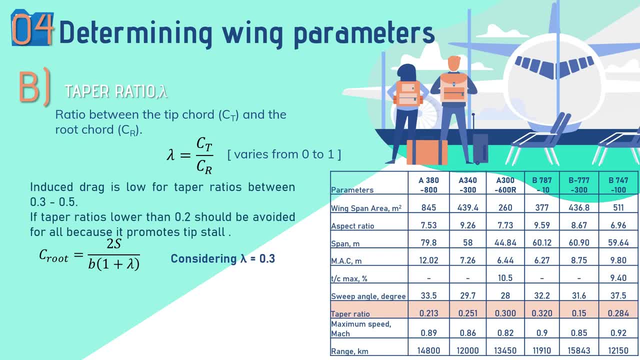 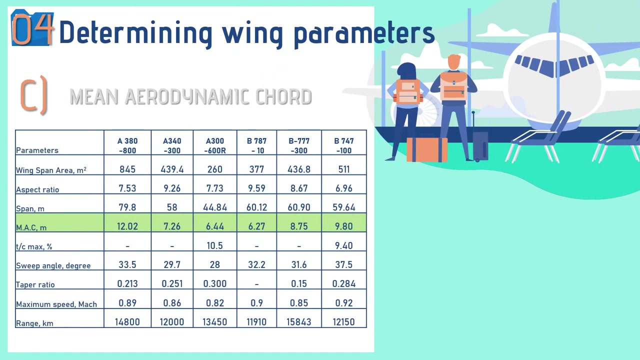 in that formula, that is root chord formula, that is 2s by b, 1 plus of lambda substituting, i have got my root chord about 10.5 meter. then substituting back to original tapper ratio formula, chord becomes lambda into c, r equals to 0.3. into 10.5 becomes 3.15 meter. the next one is to find the mean aerodynamic. 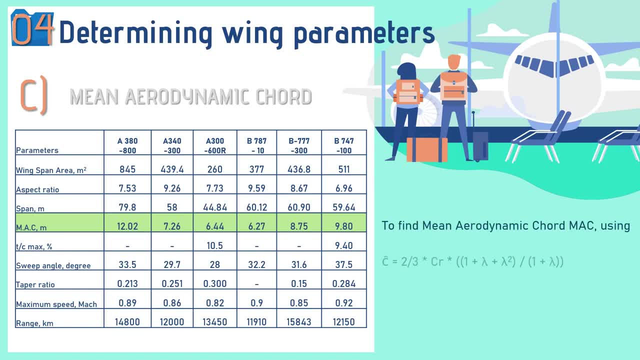 chord mac, using the formula that is, c bar equals to or c mean equals to two-third of c, r 1 plus lambda plus lambda square by 1 plus of lambda. now substituting back the values and after calculating, we got the c mean. aerodynamic chord becomes 7.5 meter and if you see the 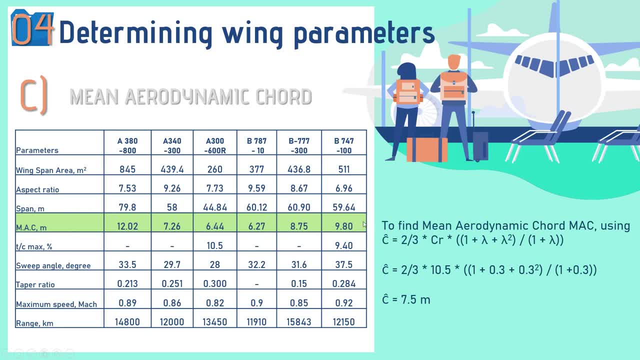 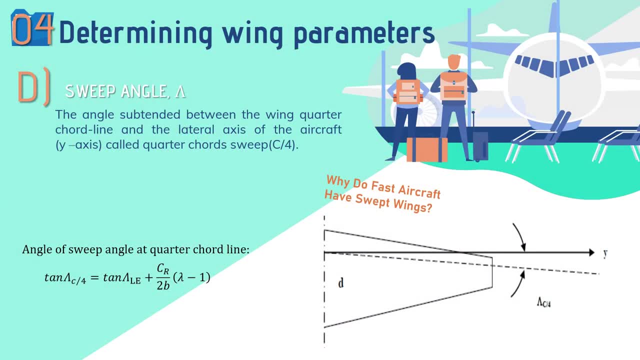 data which we have found for the large passenger aircraft and which is ranging within this 7.5.. so, moving to an next parameter is a swept angle. it is angle between the wing quarter chord line and the lateral axis of an aircraft, as shown in figure. it also affects the maximum. 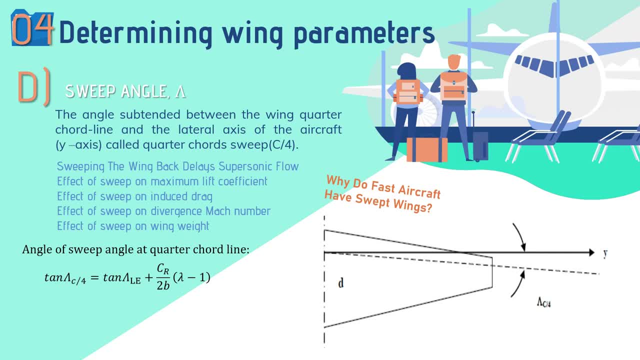 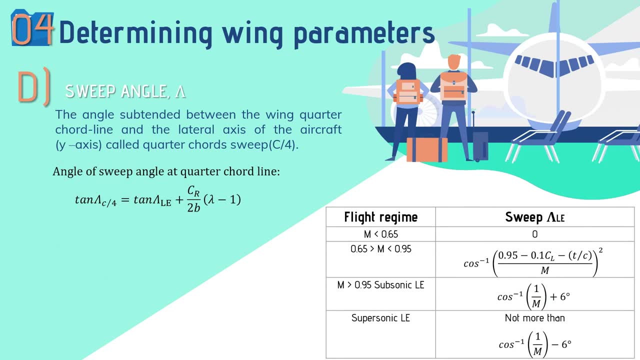 lift drag coefficient, critical mach number, structural width, stability, etc. and so on. so how to find the swept angle? find the swept angle in the following video for your aircraft now using this formula, as you can see, for, based on your flight speed, if the mac number is less than 0.65, there won't be any swap angle, but once it increases the angle, you. 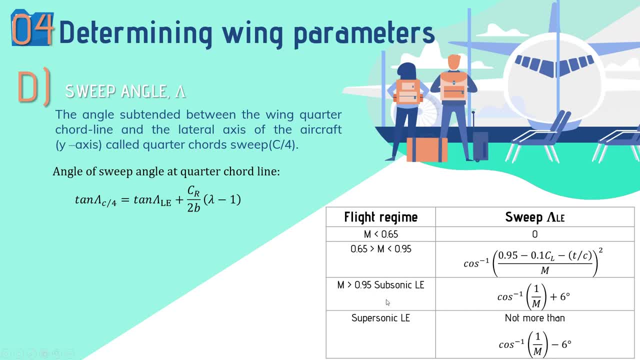 have to use. based on this formula now our mac number is about 0.85. now i have- i'm gonna use this formula now- substituting the corresponding value of my aircraft, and i have obtained this swap angle at the leading edge becomes 35.31 degree. now substituting back to the previous. 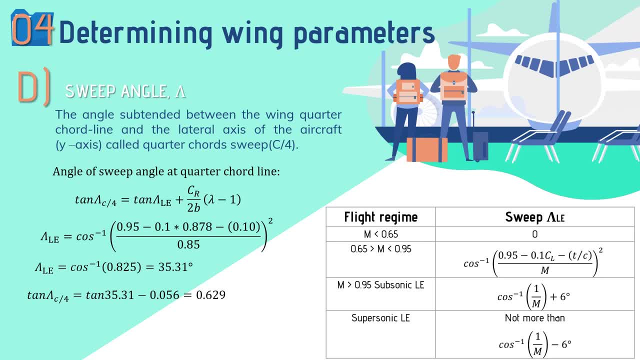 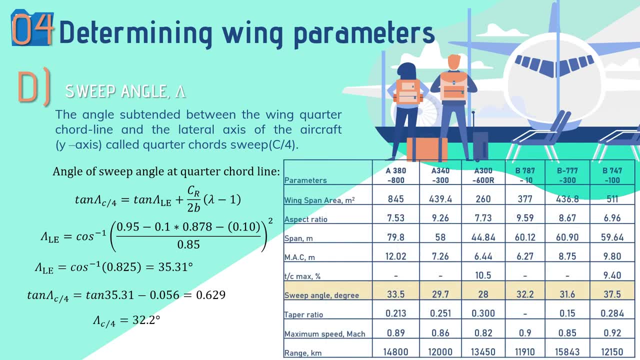 equation again, then i'm getting us that quarter chord swap angle becomes 32.2 degree. so this becomes my quarter chord swap angle. now, coming back to the reference that for my large passenger aircraft, which is ranging between 28 to 37.5. so as you can see that 32.2 is ranging within the 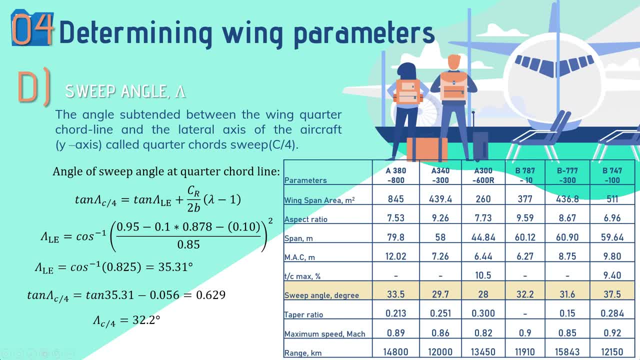 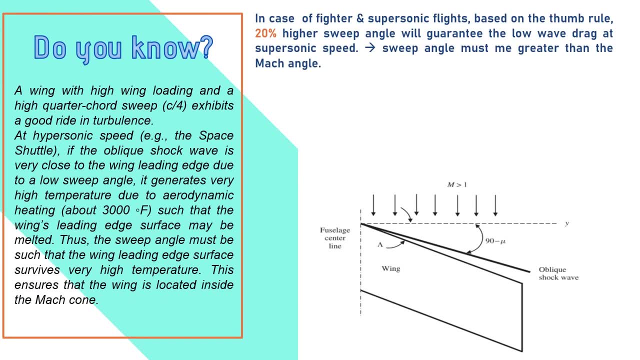 limit so that my estimation, or the calculation yet now is completely perfect. so, in case of fighter aircraft, uh, keeping that in mind, in case of fighter aircraft, the swap angle tends to reduce the shock wave, based on the proper thumb thumb rule: the 20 percentage higher the swap. 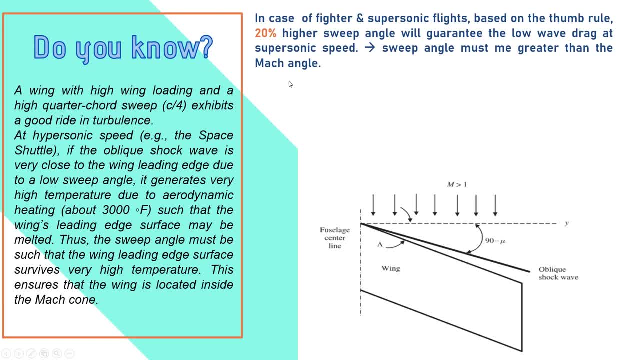 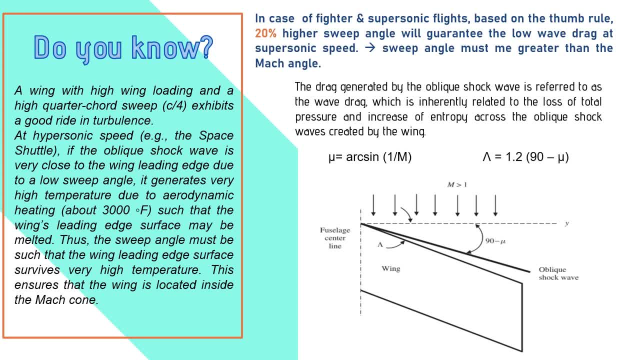 mac angle using this formula, that is, mu sine inverse of 1 by mac. once you find the mu, then substitute back over here: capital lambda equals to 1.290 minus mu and see what is the value of your lambda like how you have to satisfy your design requirement. next comes twist angle according to: 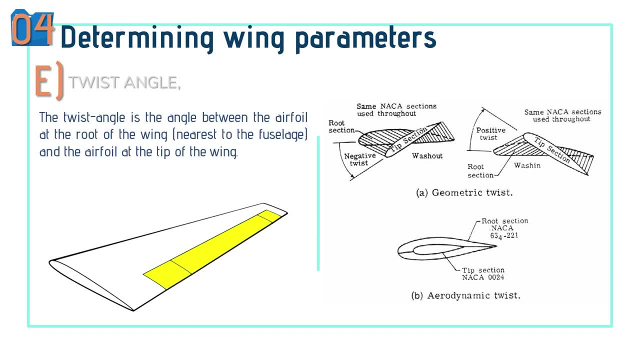 the rammer wing twist typically ranges between 0 to minus 5 degree. this number applies to an conventional wing twist angle which is 0 to minus 5 degree. this number applies to an conventional wing twist angle which is 0 to minus 5 degree. this number applies to an conventional wing. 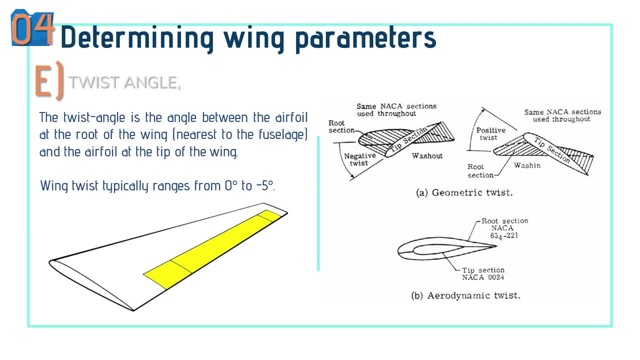 which is 0 to minus 5 degree. this number applies to an conventional wing where dial is held by the drive shaft, with a great advantage of having dynamic ponyuate. elle일�er, vous avez, see freedom. move your pvc switch on unterstütours. the cybrelocker also has gravity control on the arcaneadores. 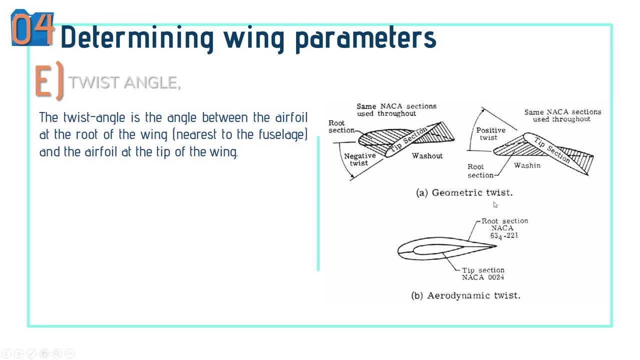 sometimes you can also Вы torture the whole test for that institute. often better to include this eines from a��따 for each test, because without the looping muito a negative angle of attack. such kind of phenomena give an wash out twist, but keeping in mind both the airfoil of same naka series. second category is a wash in, wash in means when the root airfoil 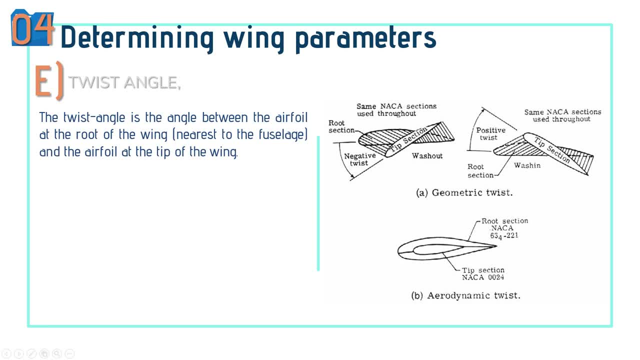 is in zero degree and the tip section airfoil of an positive angle of attack. such positive twist gives an wash in twist. but in case of aerodynamic twist both the root section and the tip section are different airfoil section. it can be, as you can see in the figure, that root cord section. they 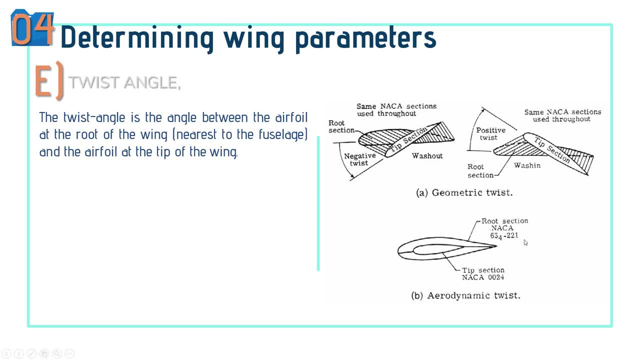 have considered naka 3, 6, 3, 4, 2, 2, 1. the thickness is around 21 percentage, whereas the tip section they have considered the naka 0, 0, 2, 4. that means thickness is 24 due to the difference in airfoil. 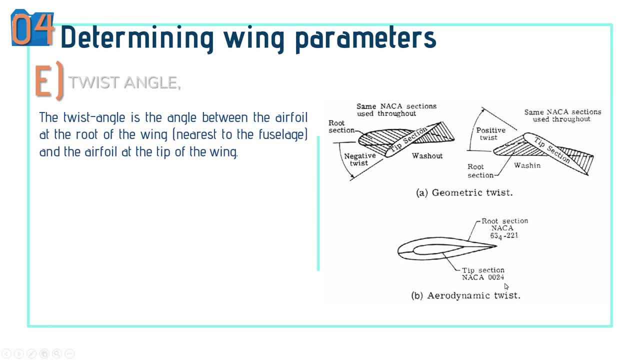 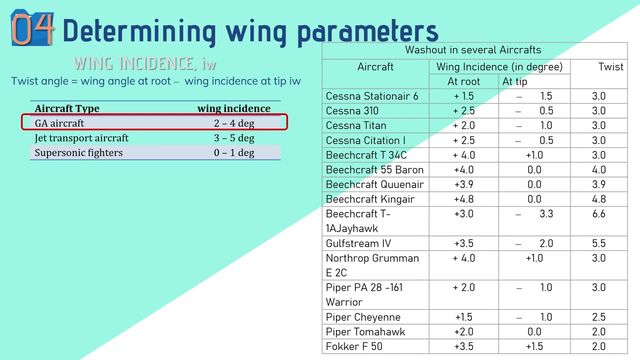 in the root section and the tip section, it created an automatic twist. such twist is known as an aerodynamic twist and it leads to an wing incidence that is iw so and the twist angle is equivalent to the wing angle at tip and the wing incident at the root. so, based on this criteria, based on your design, 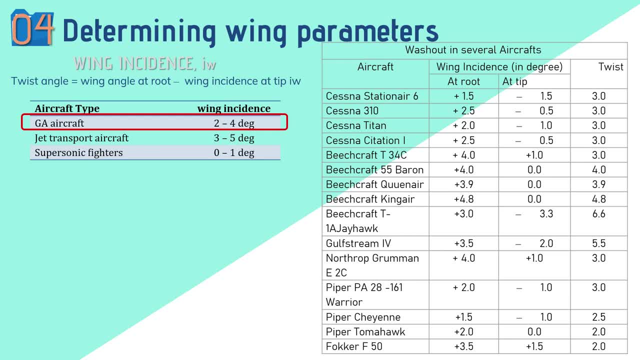 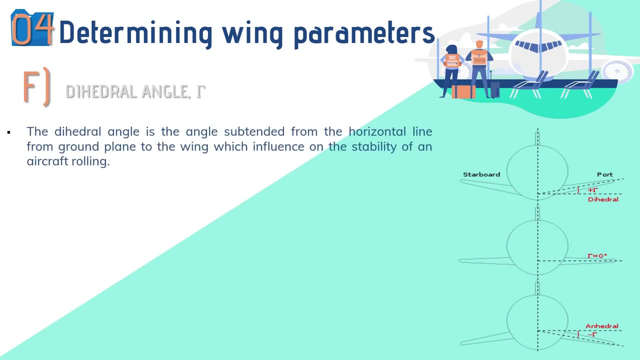 criteria or the reference table, you can choose a proper angle of incidence for your design aircraft. so, mostly for my design, i will consider the two degree angle of incidence, not more than that. so coming to the next, is an dehydrael angle, is an angle subsたnded from the horizontal line or from the ground plane? 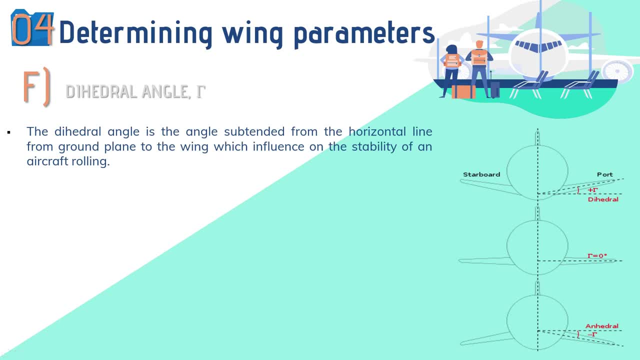 to that wing which influences on the stability point of view. so here dehydrael also plays an important role, based on the placement of the wing of a fuselage, so the mostly the wing tends to have considerably greater dehydrial angle than the high wing. so for 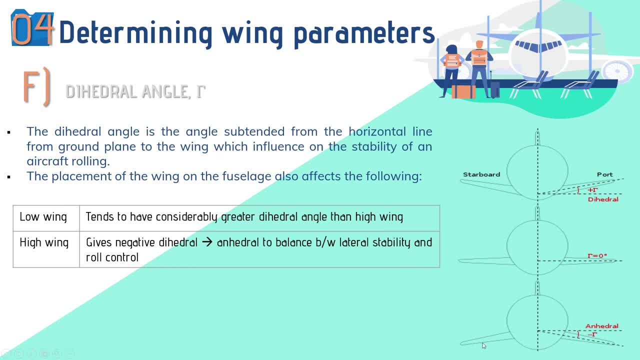 an example for the passenger aircraft and high wing gives a negative dehydrale angle, angle which is called as an anihedral, to balance between the lateral stability and the roll control. so, based on the parameters are displayed for a high wing, 0 to 1 and for low wing even 3 to 8 degree. it can be considered so based on. 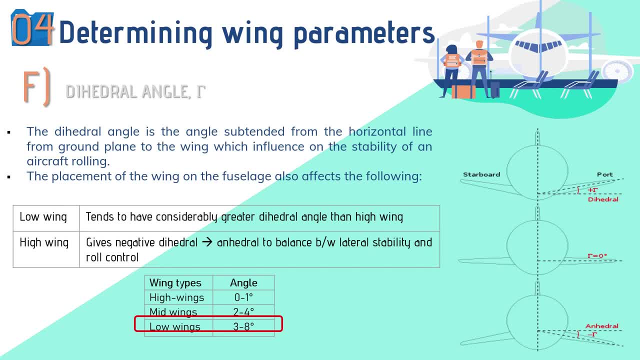 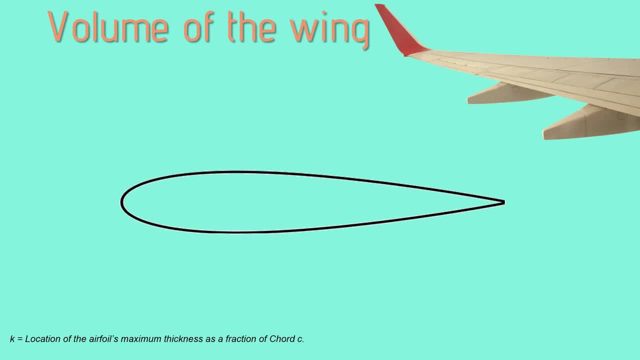 your type of aircraft, you can select the best parameters for your design. coming to an most important factor is an volume of wing. so often, the cross-sectional area of an airfoil must be calculated using some clues about an internal volume of a wing available for an fuel storage right. so, based on the internal 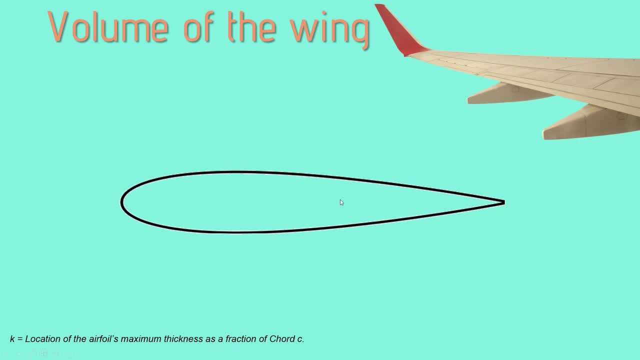 geometry estimations. so first, what we'll do is we'll split the airfoil into section. first is an parabolic section and second is a triangle section. so the parabolic section will be splitted from the position of maximum thickness point of the chord and remaining will be the triangular section. so as you can see so, 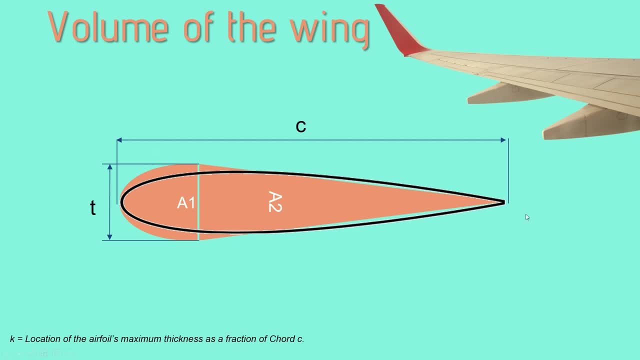 we have given some nomenclatures of that particular phenomena. the length of the airfoil is C and from the section K is the location of maximum thickness of the chord and remaining is 1 minus of K of C and thickness is T. you can see there. so 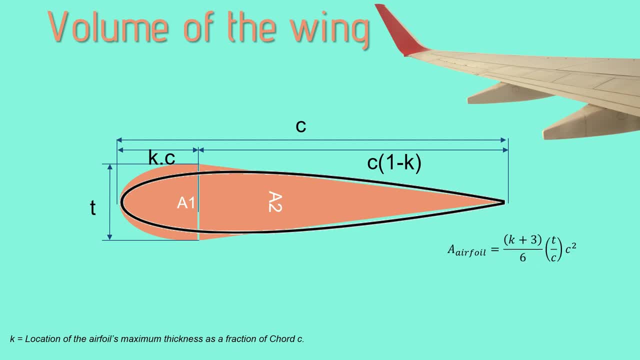 we will get. the area of the airfoil becomes K plus 3 by 6 by T by C of the C square. so this is the formula for the volume of an airfoil, that is B into C R square by 12 K R plus 3 T by C of R plus K T plus 3 T by C of T lambda square. now 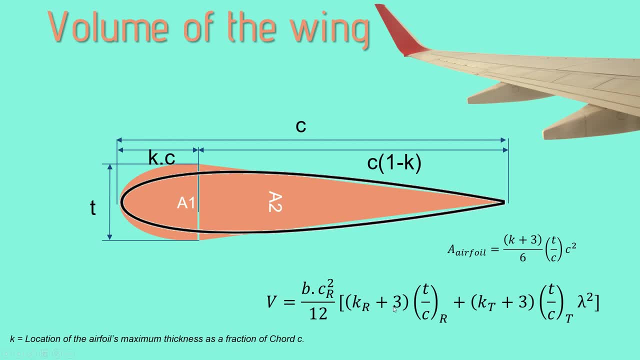 all the suffix of R represents that root section and T suffix represent the tip section. now NACA SC series and in that series we have the 10 percent of thickness and 38 percentage of the chord at the 38th percentage of the chord. so that means around 0.38 of the chord right. that is K, R becomes 0.38 and T by 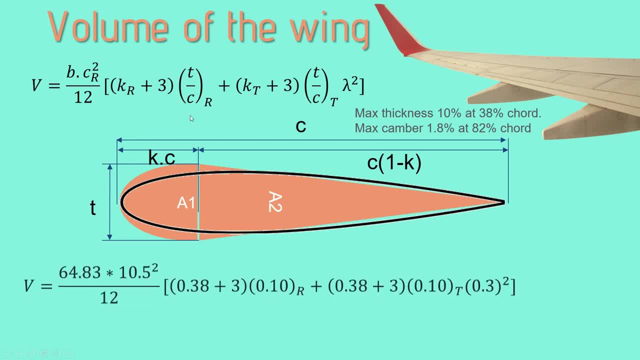 C becomes 0.10 now substituting back in this formula, and B, what we have calculated is 64.83 and C R value is 10.5 now based on the formula after substituting and we are getting the value about 21.44 meter cube now, recalling that in my last lecture we have considered that 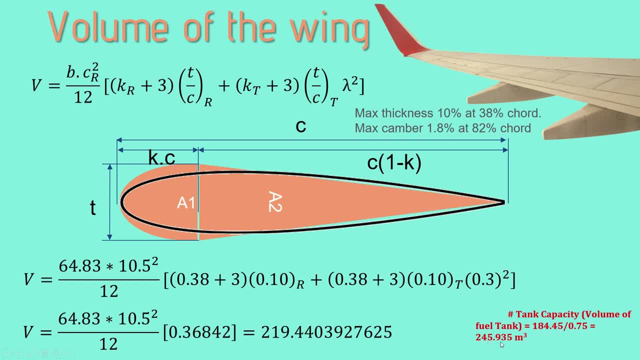 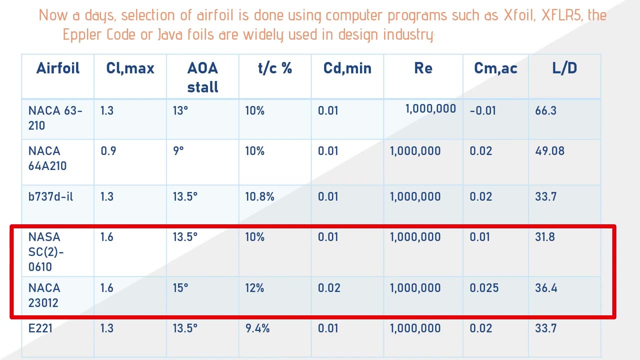 tank volume capacity came around 245.935 meter cube, so that means the volume which I'm getting is less, and that won't satisfy my requirement. now what I'm gonna do is this design is not satisfying my requirement, so I need to make some changes. so I will show you the 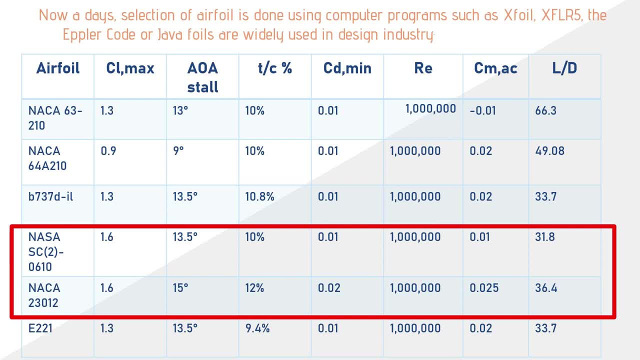 changes which I made. now I will go back to my selection of airfoil. now, in that selection of airfoil, what I'm gonna do is I'm going to select. now I'm going to do a minute change in my airfoil design. the change is that in the root chord I 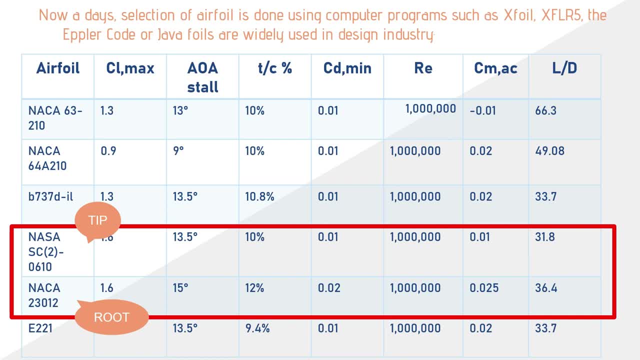 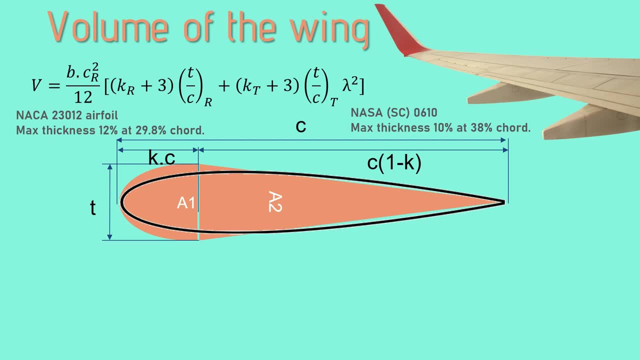 will consider NACA 23012 and the tip. I will consider NACA SC20610 now here, each having its own parameters. that for NACA 23012 it is in 12 percentage of thickness and root chord is 29.8 percentage of the total thickness. 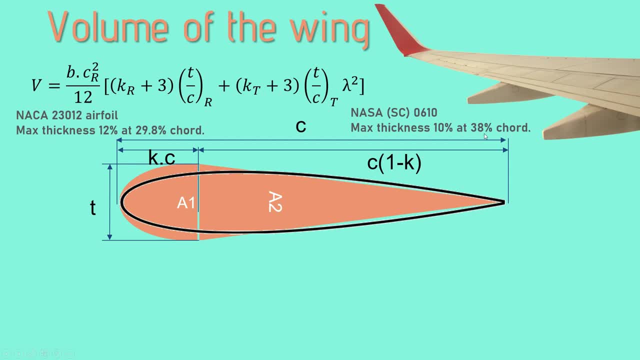 and in case of this is 38. so using this formula, okay, the total wing volume can be opted. so where lambda becomes tapper ratio and k becomes a location of airfoils, maximum thickness as a fraction of chord and the subscripts of r and t refers to that root and the deep airfoil maximum. 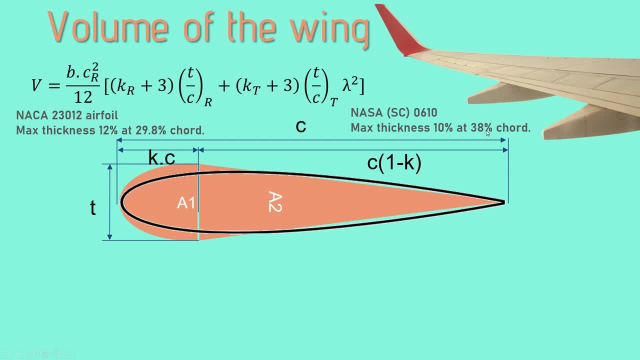 thickness at percentage of chord. okay, so in case of 23012 it is 29.8 percentage of chord. that means point k value is about 0.29, but in case of for the tip it becomes 0.38. now substituting back in this: 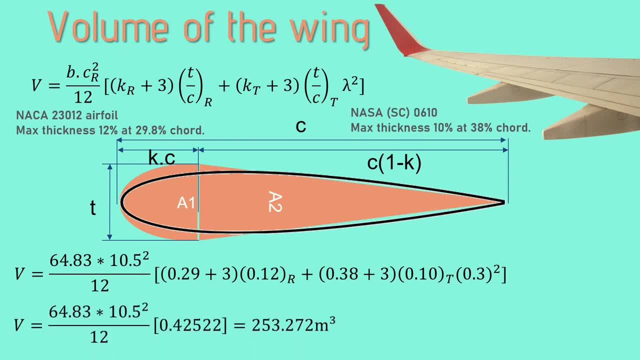 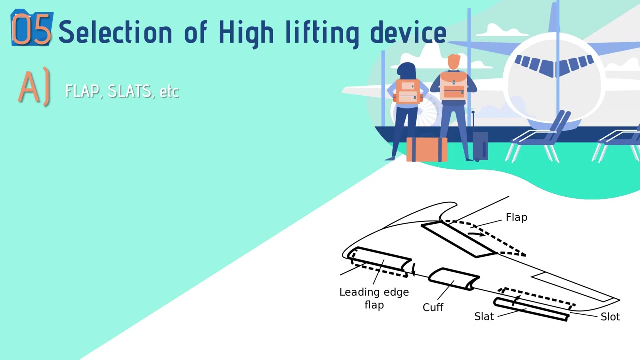 equation again and rearranging the form: okay, and where i am getting the value about value, about 253.272 meter cube, and now it is, you can conclude that it is satisfying the volume of my fuel tank. so i can proceed further. now i will proceed with an selection of high lifting device. now, high lifting device are the movable surface. 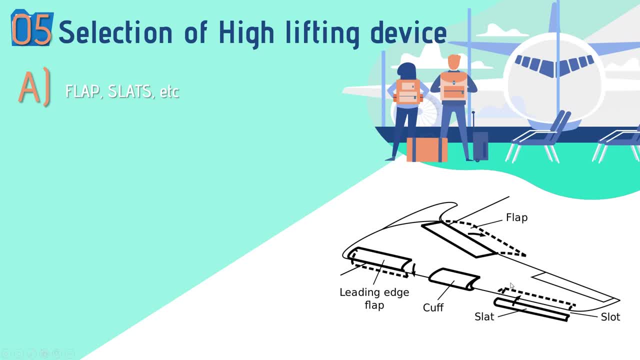 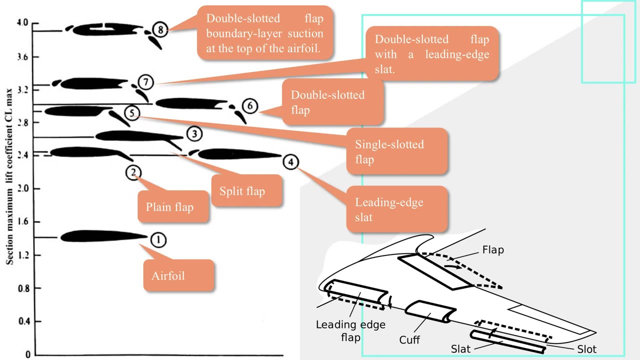 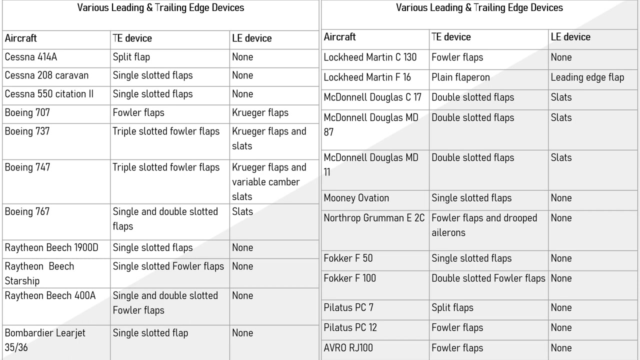 or mostly used during takeoff, takeoff and landing. so most commonly high lifting device are flaps, slats, right, etc. so here are few of the types, common types of flaps and slats, by comparing the various type of flaps, each flaps having its own lift increment and with an application. so 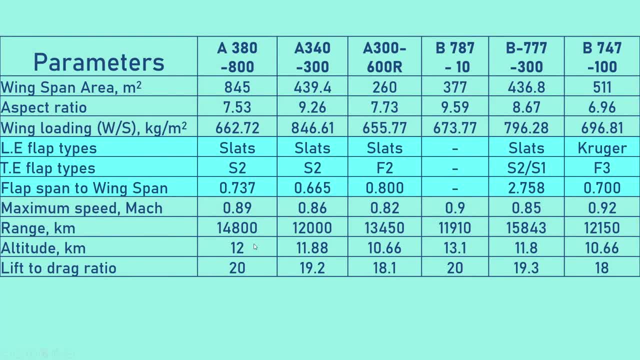 our type is an jet transport. so here in my design i will compare few datas. here are the basic examples as well as these are the comparative data which i have found for my design table, for my design parameters. so mostly they have used uh slats as a leading edge flap. 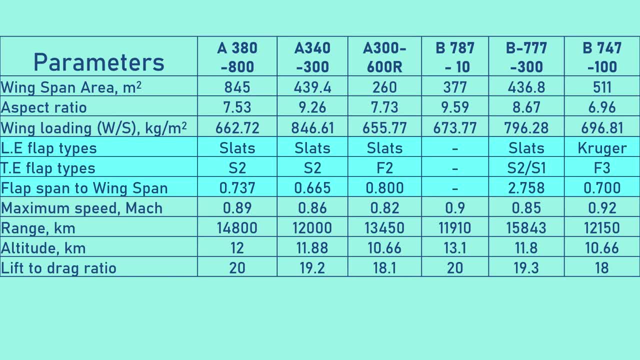 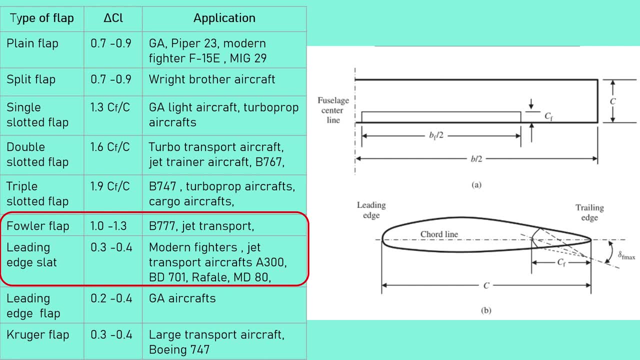 and trailing edge. they have used double slotted flap. so but in case of my design, i am going to choose a fouler type. p77 jet transport using fouler type with this leading edge slat. you can also select your type of design. you can also select your type of design. you can also select your type of. 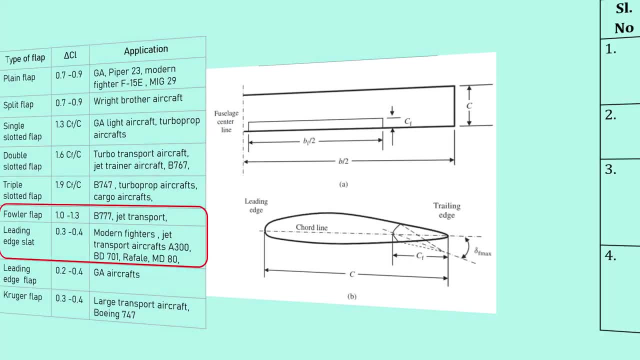 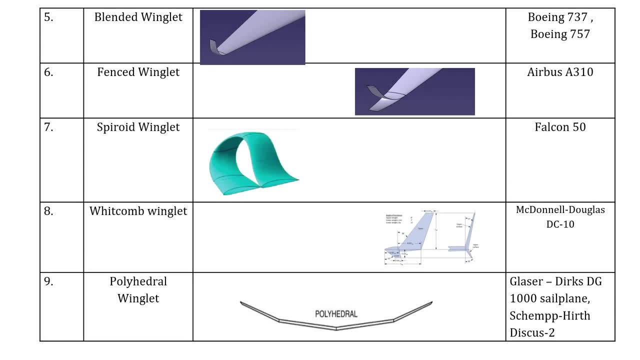 flap based on your design criteria. moving to the next is a wing tip now wing tip off of several types you can see right now here i will use a blended wing type of for my design criteria, because boeing 737 and 757 are mostly used as a blended wing, uh, winglets, and it is also. 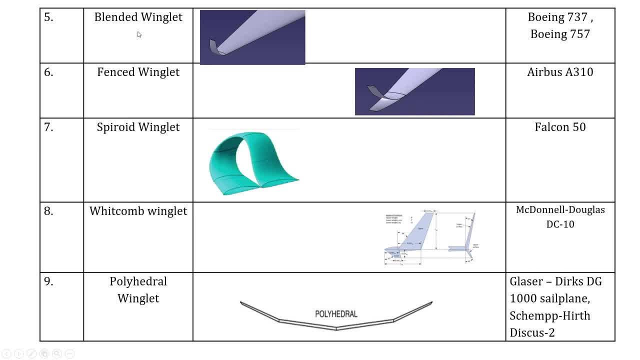 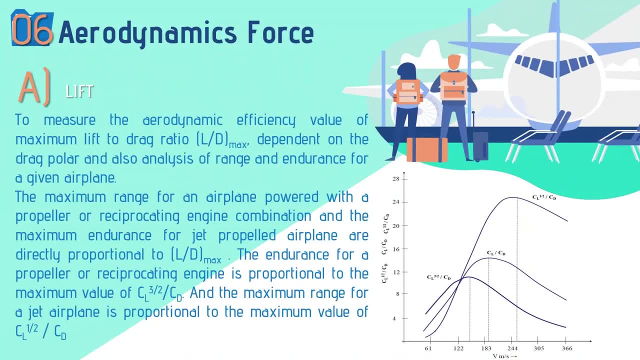 configured very simple, not like with a fenced winglet. so this is also my type and, based on your configuration, we can select the type of winglets. now coming to the next is an finding out the lift forces. okay, to measure the aerodynamic efficiency, the value of lift coefficient to drag depends on 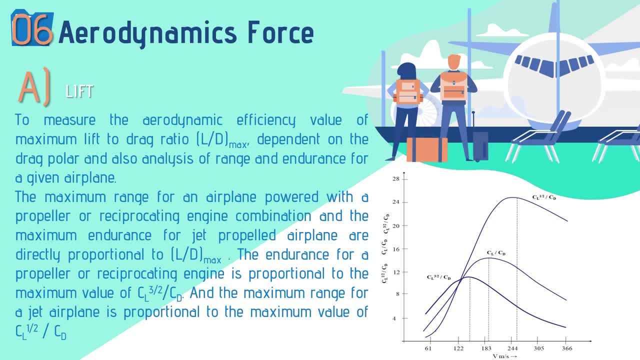 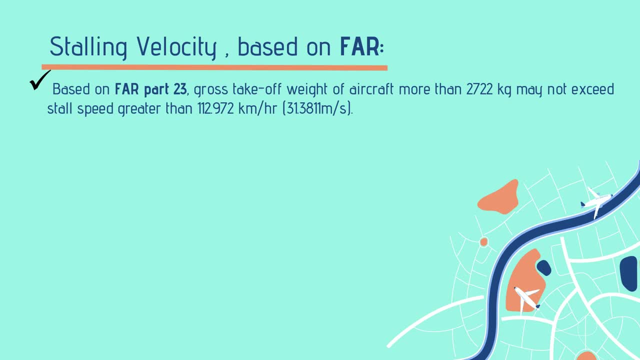 the drag puller and analyzing the range and endurance of an given aircraft. so first proceed with an stalling velocity based on far. so, based on far, part 23, the gross weight of the aircraft, 2722 kg, may not exceed the stalling speed greater than 31.38 meter per second. but in case of light, 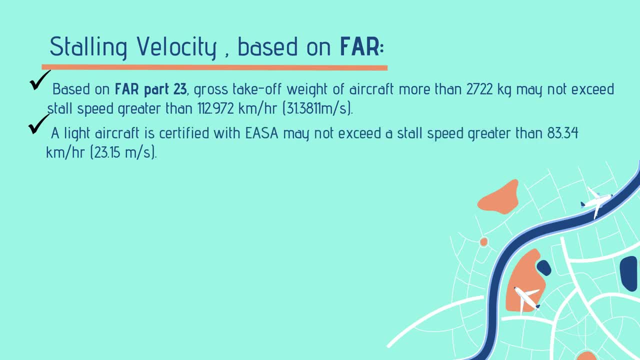 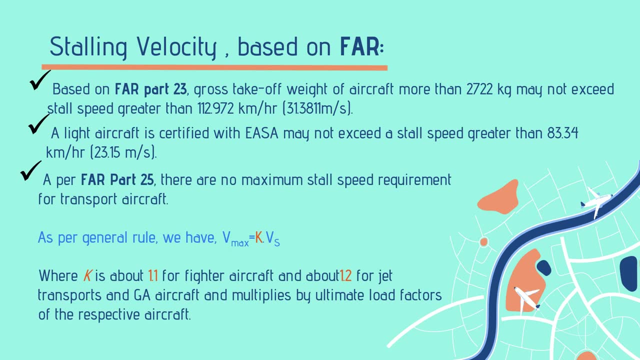 aircraft, like gliders and all, it should not exceed more than 23.15 meter per second. but in case of today's, our design is about large passenger aircraft or any fighter aircraft. there are no maximum stall speed requirement for an transport jet, so as per the rule we have, v max equals to kvs. 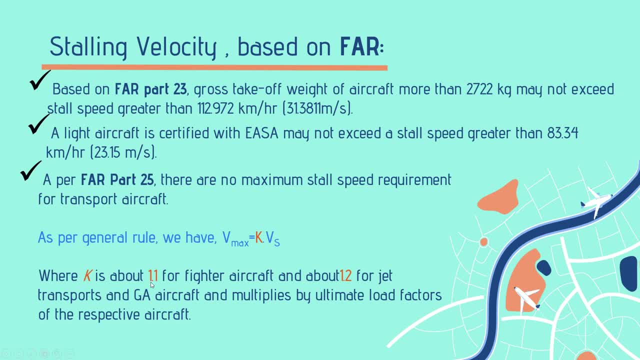 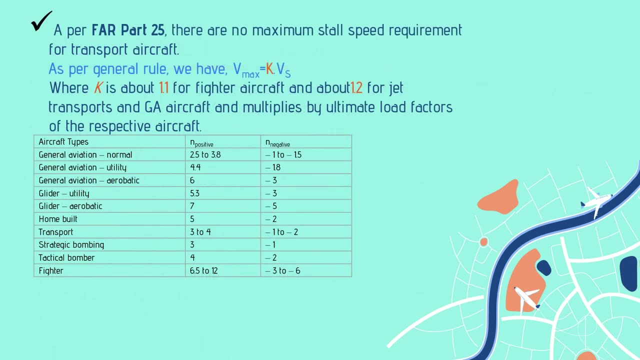 now k is the value or the factor depends on type of aircraft. in case of fighter, you need to multiply 1.1 and in case of jet transport and aircraft need to multiply 1.2. in addition, multiplying by ultimate load factor of a respective aircraft- in my next slide you can see: 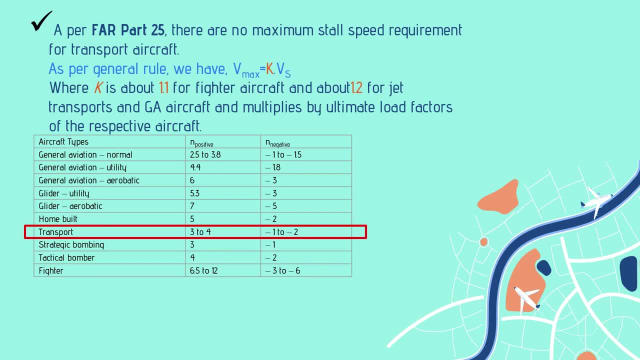 that uh foreign transport jet which we are designing over here, which i am designing over here. it's about maximum ultimate load is 4.. now i will multiply that with terms. that is 290 by 1.2 into 4, so where i get my stalling speed as 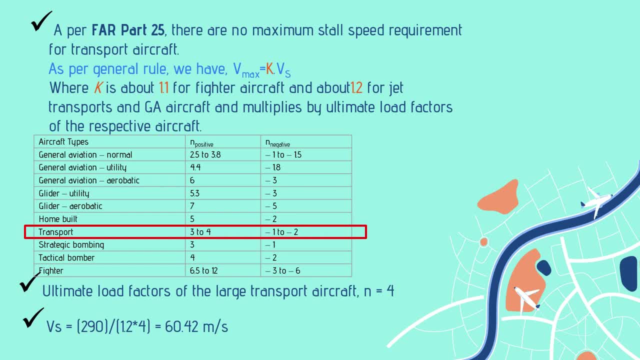 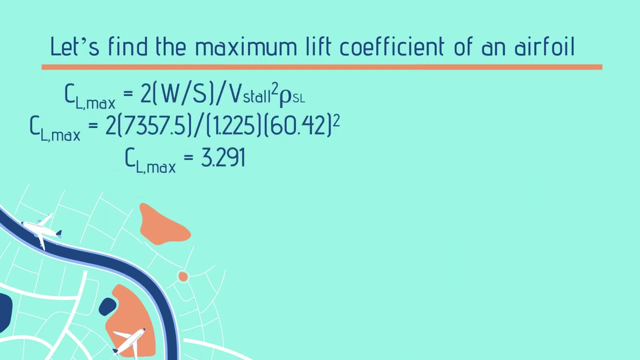 60.42 meter per second. so, based on your type of aircraft, you can multiply with an ultimate load factor for your design aircraft. proceed with the next is that to find out the maximum lift coefficient of an airfoil. so for cl max becomes that 2 w by s v stall square, rho at the c level. 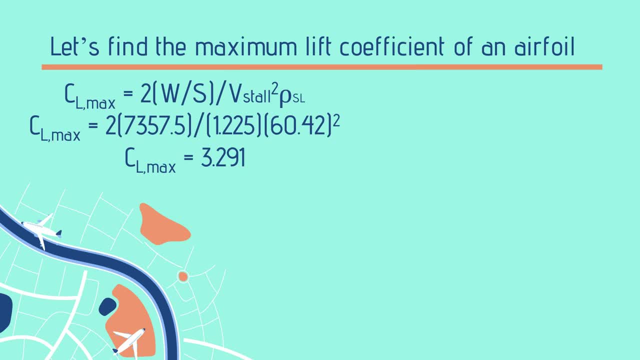 now substituting the values of wing loading is 7357.5, rho at c level is 1225 and v stall just obtained that is 60.42 square. now substituting back, we get that maximum cl becomes 3.291. now for the wing, similar fashion, we will find that cl max. 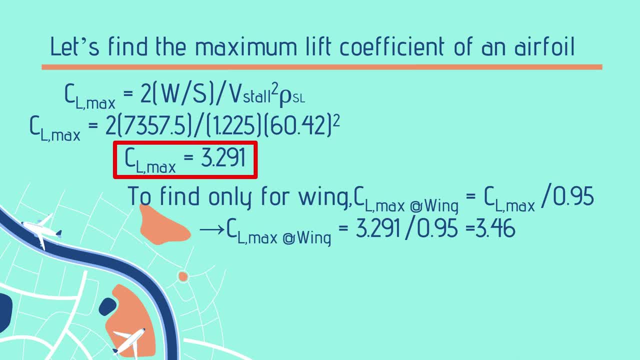 by 0.95, we get as 3.46, and for the airfoil that is divided by 0.9, we will get as 3.85. now, recalling that we have selected here is a follow type, which is when it is fully deflected. 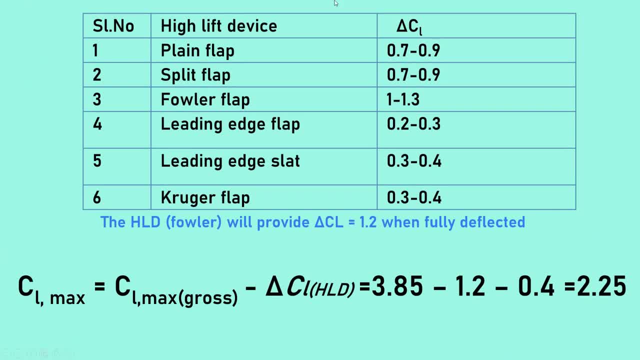 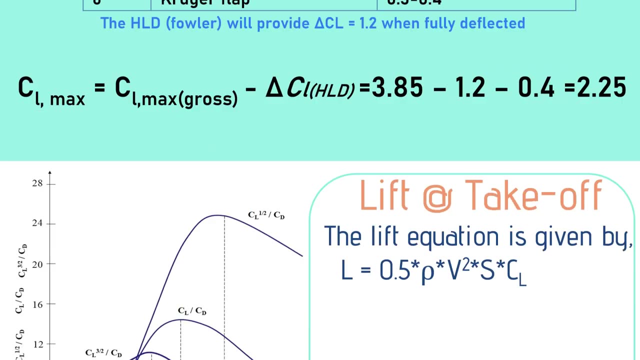 and the slot type. now to find out the cl max, there is a cross value which we have obtained without that high lifting device, so we will get that actual. we will get, as on, 2.25 without the high lifting device. so now recalling back lift force during takeoff: now we know the proper values. 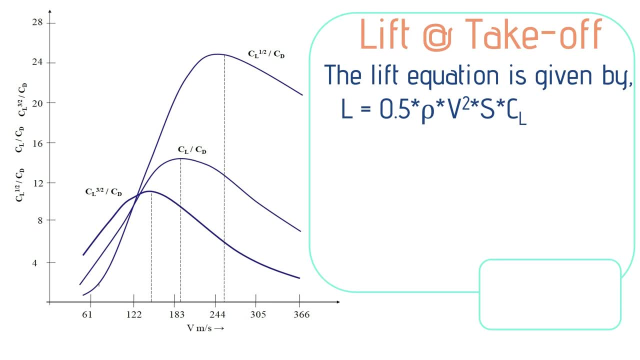 that is half rho. v square scl density at the c level is 1.225 kg per meter cube for a general aircraft can be fined using 1.2 of v stall. v stall is 60.42 into 1.2 you will get 72.504. 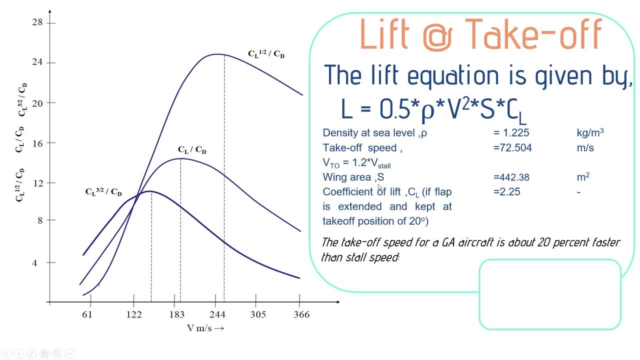 now wingspan area is 442.38 and the maximum deflection is on 2.25, as we have obtained right now. so using this formula, we will get substituting back to the original formula and get us 3204852.35. now coming to the next. 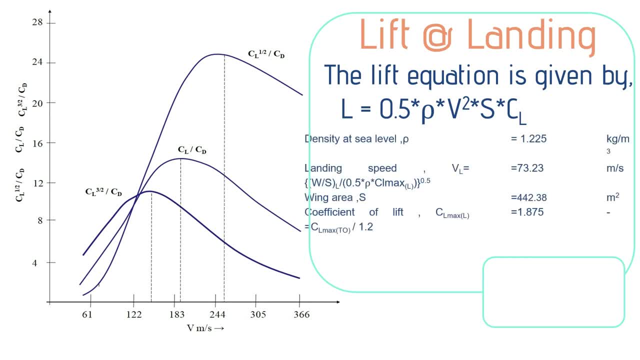 similar fashion we will find for the landing. for landing here you have to carefully choose the landing speed. so using simple formula that is, w by s of landing, that half row cl max- okay for a general aircraft landing weight- should be equals to 0.85 a total takeoff weight. so using the parameters we 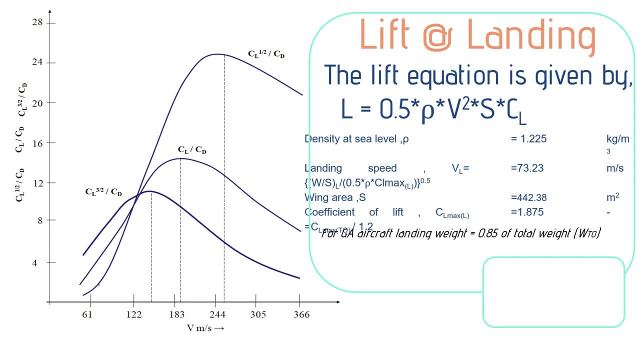 have to find out the weight of the weight of the aircraft during landing. substitute there then the lift coefficient for landing. that is, divided the total takeoff weight divided by 1.2, we will get as 1.875. now substitute all the parameters in the previous equation and you will get 2724463.021. 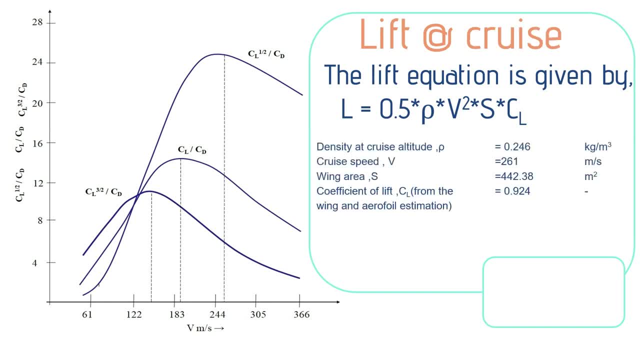 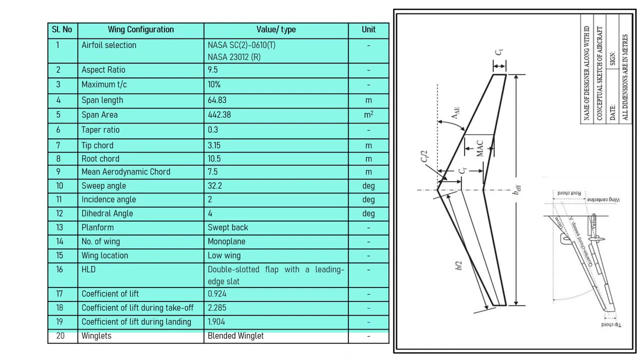 Newton for the cruise. we have already found out that lift coefficient value. just you need to substitute to find out the lift force and we will get around 33598708.8 Newton. and finally, you will write down all the parameters for your aircraft which you have finally chosen and optimized and further you.